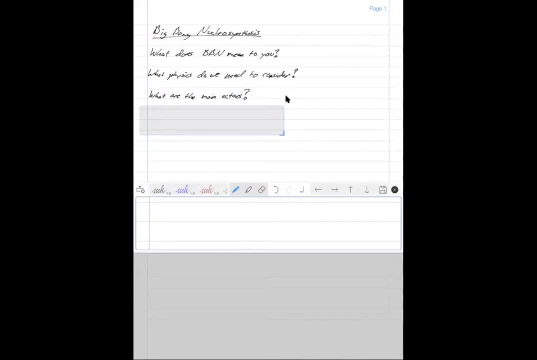 questions. So what does Big Bang Nucleosynthesis mean to you? So for some of you, this, you might say, is a nuclear synthesis. So what does Big Bang Nucleosynthesis mean to you? So for some of you, this, you might say, is the synthesis of nuclei at high temperature. This is associated. 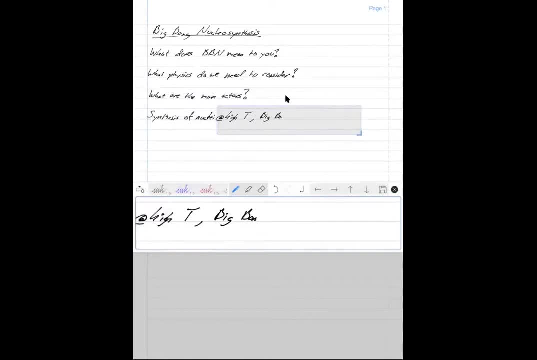 with Big Bang And maybe this is nucleus synthesis in the high entropy regime. Maybe some of these are the answers that came to you, But one thing I really want to emphasize is that this Big Bang Nucleosynthesis is really at a process of freeze out. We start out, we're 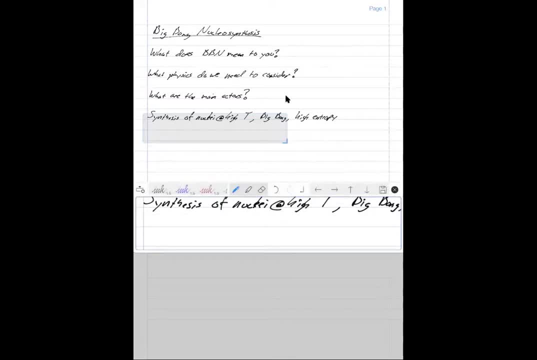 going to start out with free neutrons and protons and consider all the possible interactions during a certain time period And as the universe expands and cools, we're going to be looking at freeze out. In particular, Big Bang. Nucleosynthesis will predict that roughly 70% of the universe is hydrogen and 30% 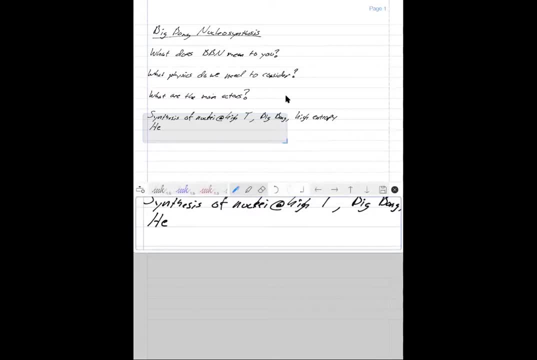 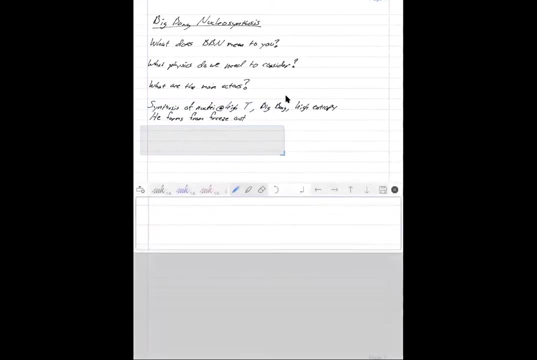 is helium And there's trace amounts of everything else. So helium forms from freeze out. So that's one thing I really would like you to remember about Big Bang. Nucleosynthesis is that it's really about freeze out of nuclei from individual, the individual constituents of 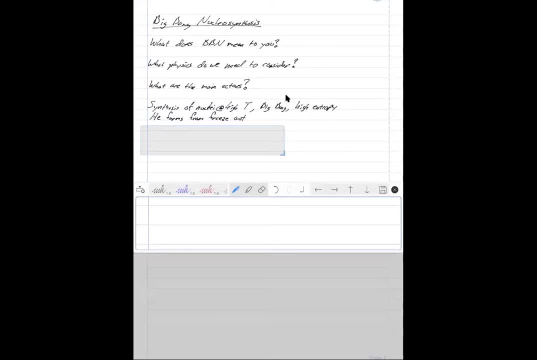 them All right. So what physics might be relevant? Well, we're going to be looking at a little bit of statistical mechanics. E and M is certainly important. We're talking about nuclei, so probably the strong force, But it turns out it's really the residual. 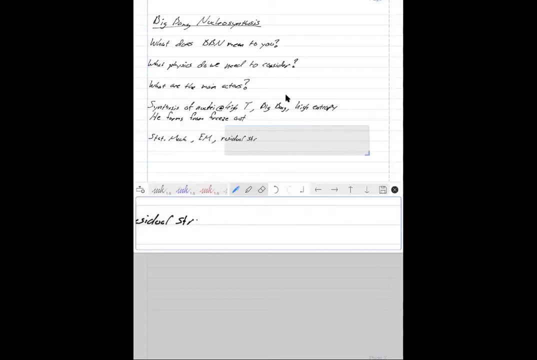 strong force. that's relevant, And we're talking about interactions within the nucleus, And so the weak force is relevant as well. Now, what about the actors? Well, there are many possible actors. Some include neutrinos. There are many possible actors. Some include neutrinos. There are. 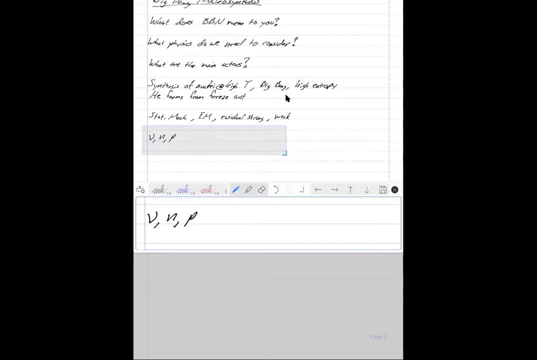 neutrinos, Neutrons, protons, electrons, positrons, and then maybe some mediators like photons, W, Z, boson. We're eventually going to form nuclei, so maybe helium-3.. Heavy metals: Heavy metals, Heavy hydrogen or deuterium. 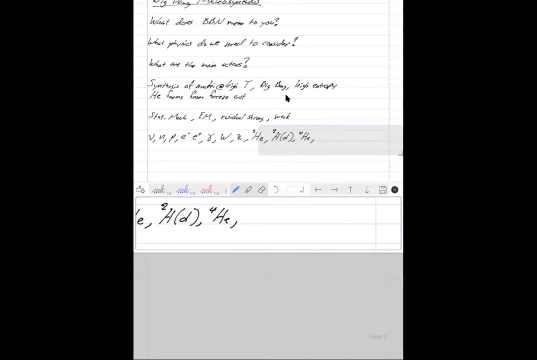 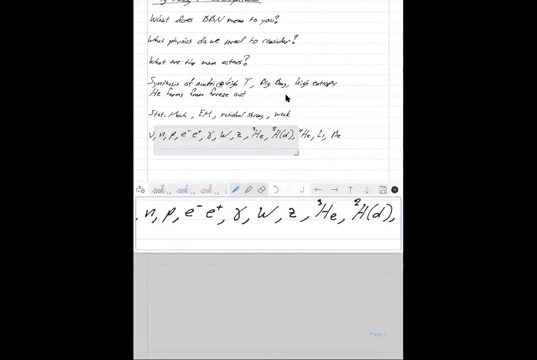 Helium-4.. Lithium, Beryllium, And these are all possible important actors. So what we're going to do in developing this theory of Big Bang Nucleosynthesis is: we're going to focus. we're going to first focus on these because they set the stage. 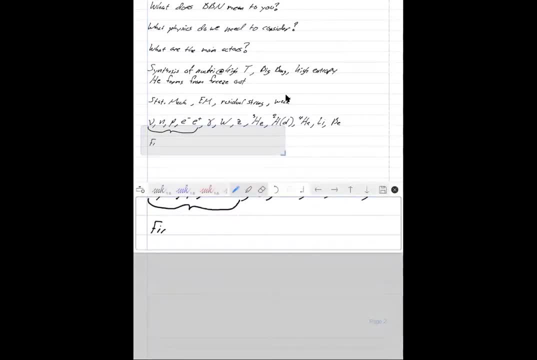 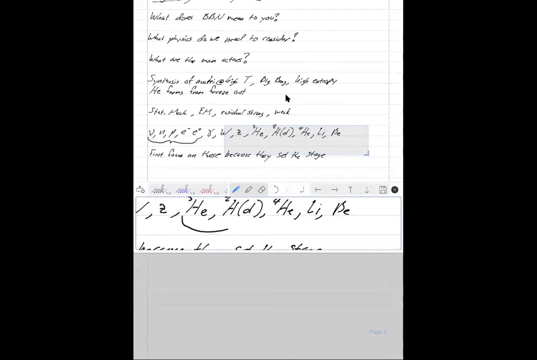 we're going to focus on these because they set the stage. So first focus on these. First focus on these, Then the bumblebees, Then the peacock, Then the Neutron, Then the, Then the Neutron, the light nuclei on the periodic table of elements. 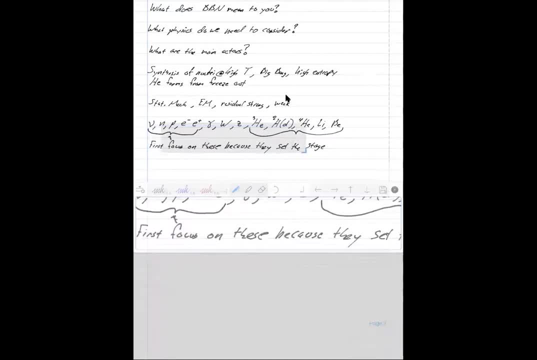 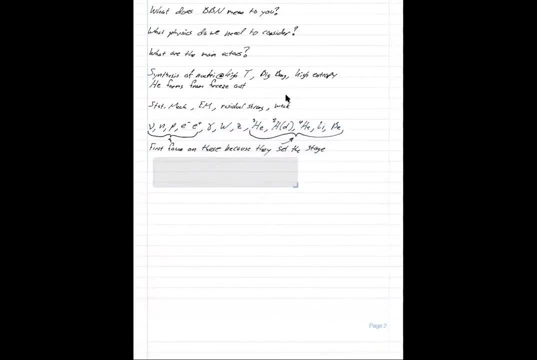 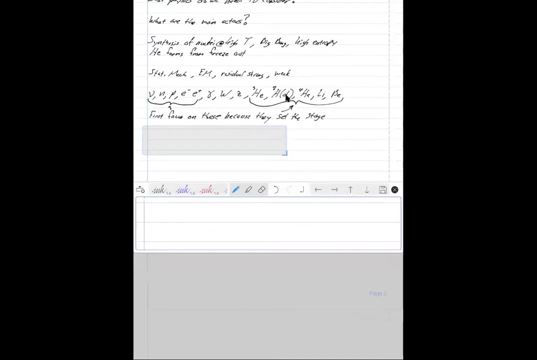 So first these to set the stage for these. Okay, And in particular, we're going to focus on three possible interactions between the neutron and the proton. So, first of all, the neutron can capture an electron-type neutrino. It'll produce a proton and an electron. 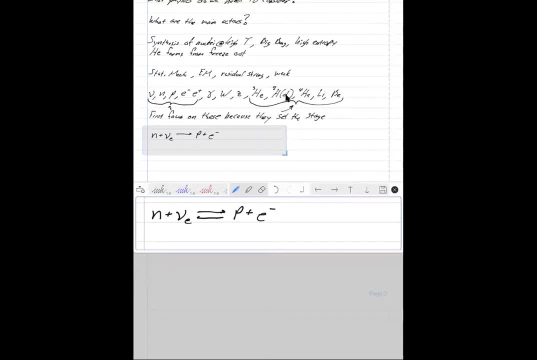 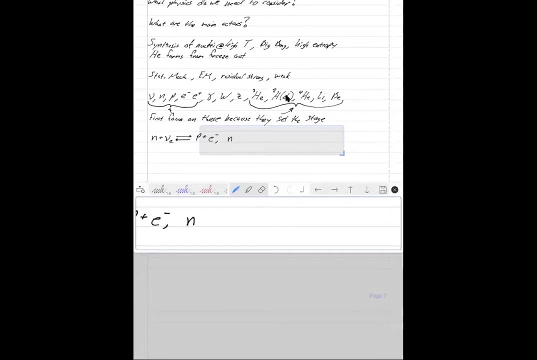 Now this reaction can go in this direction as well. The proton can capture an electron to produce a neutron, And the electron can capture an electron-type neutrino. Here's another interaction that's important: The neutron can capture a positron And it will produce a proton and an anti-electron-type neutrino. 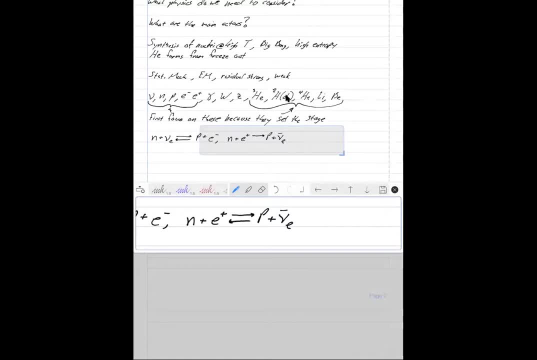 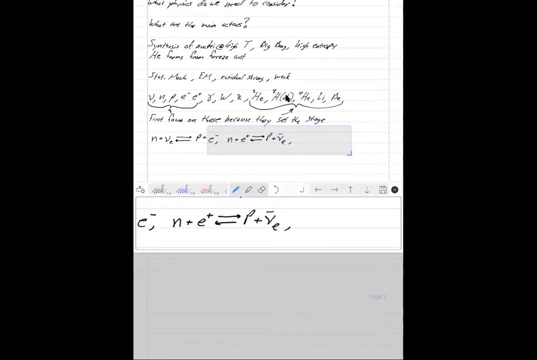 And once again this reaction can go in both directions. And then here's the third that we're going to consider in setting the stage. We can have a neutron decaying into a proton, but we need to conserve charge. And we're going to conserve lepton number with a neutrino. 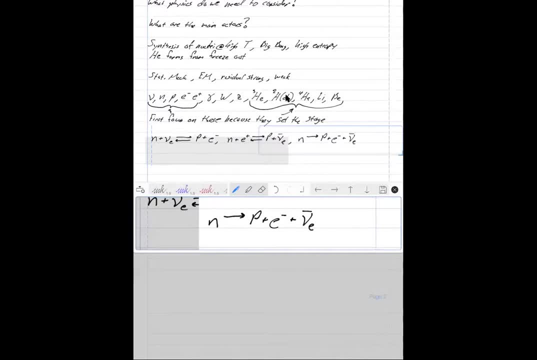 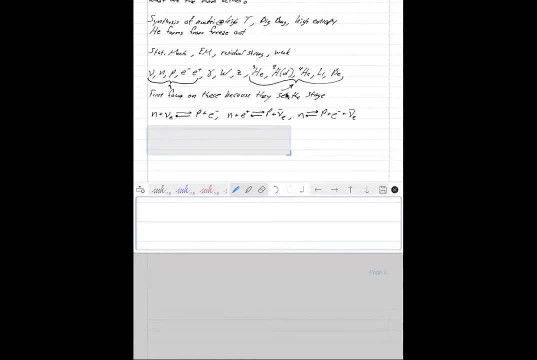 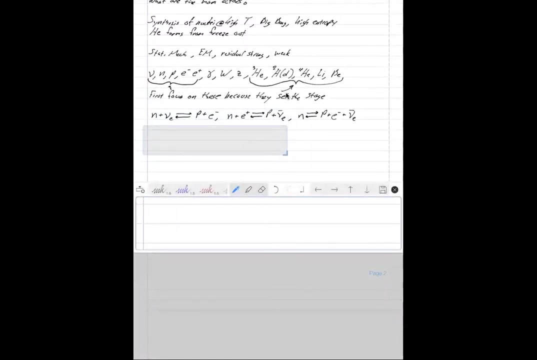 So we have an anti-electron-type neutrino And once again this reaction can go in this direction as well. Now the energies of these reactions is important. So there's an important. We notice that here the energy of the electron minus the energy of the neutrino. 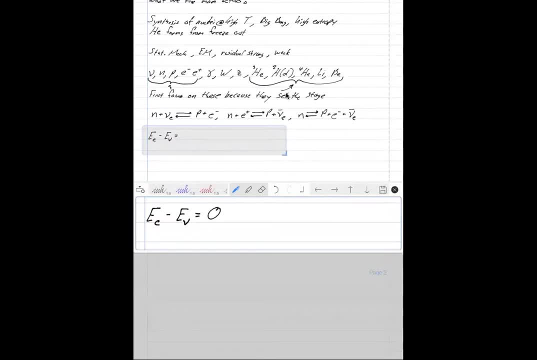 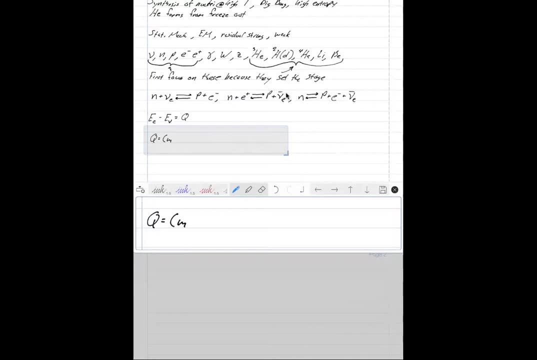 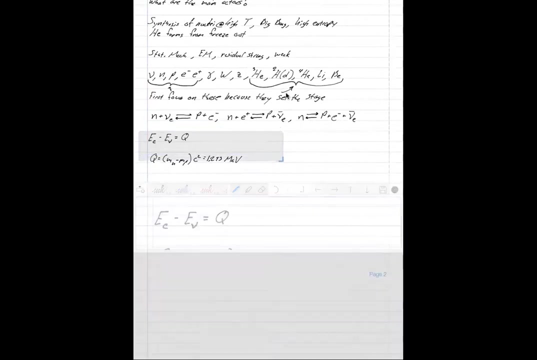 is going to equal Q, where Q is the difference in the rest mass energy of the neutron and the proton, C squared, And this is equal to 1.293 MeV, just to give you a scale for this. So this difference in the neutron and proton, 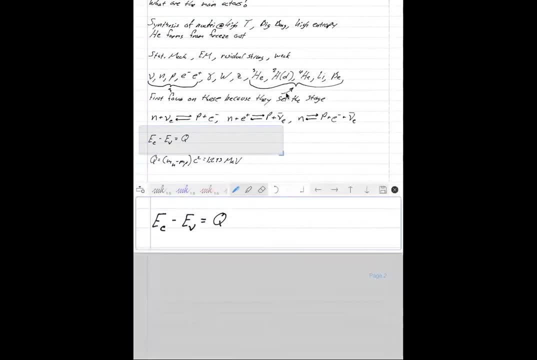 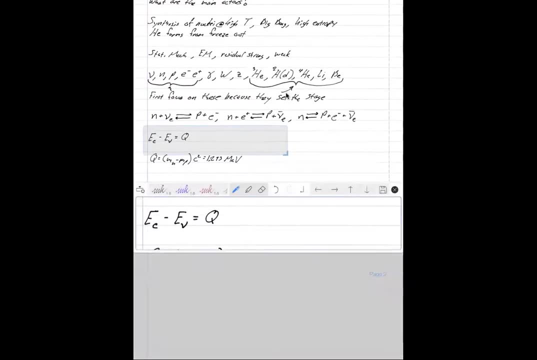 is equal to the difference in the energy of the electron and energy of the neutrino, And so those energies obviously include rest mass plus the momentum component of that. For this middle one, we have that the neutrino energy minus the electron energy is. 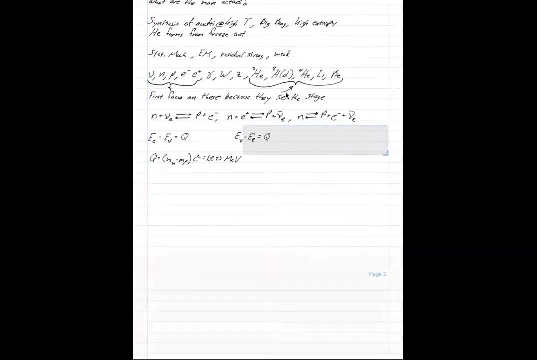 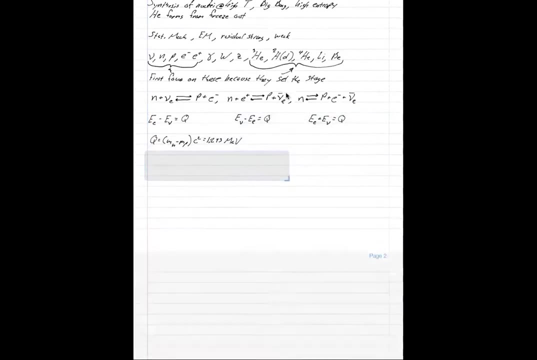 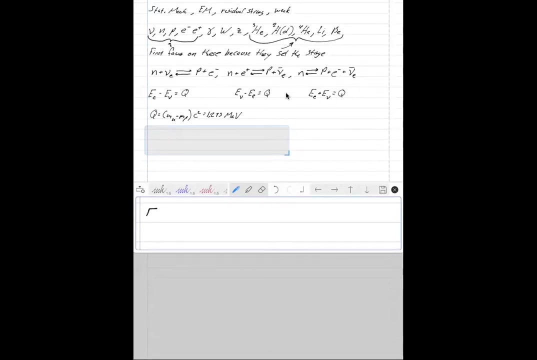 is equal to Q this time, And in this last one we have that the energy of the electron and the energy of the neutrino is equal to Q. Now for pi, temperature and density. these processes go in both directions, In other words. 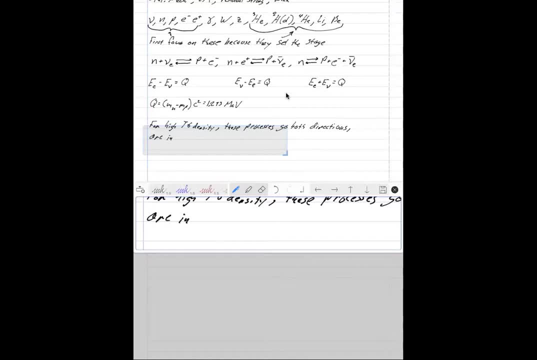 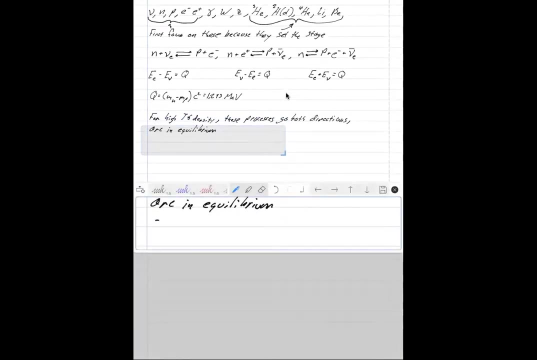 they are in equilibrium. We're going to use that a little bit later to find an algebraic expression And we're going to use this. One may derive the fraction of neutrons at any given time or temperature. Let me just put capital T. Or temperature. At some point these reactions will freeze out. We won't be able to have these reactions anymore And at that freeze out. after this freeze out, the number of free neutrons at freeze out determines the helium-4 composition. 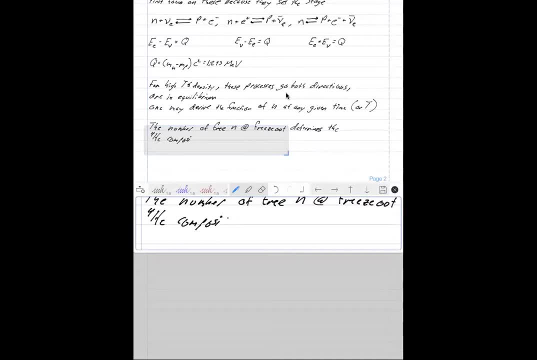 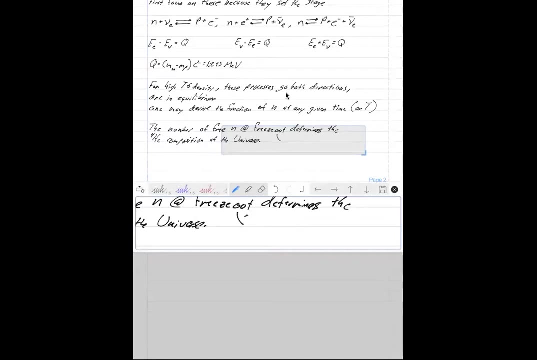 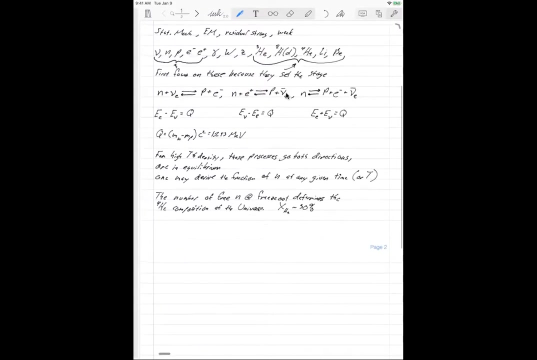 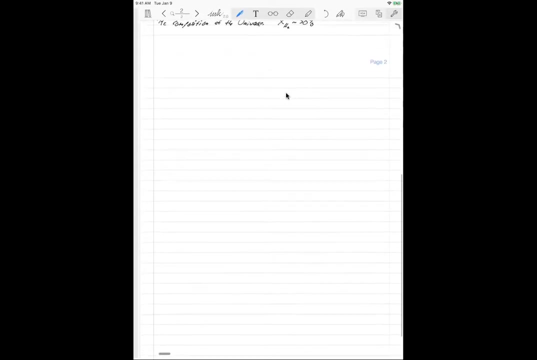 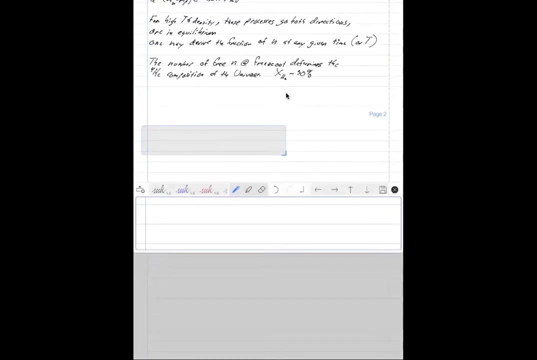 of the universe, And we're going to find that the mass fraction of helium is roughly 30%, Just from working out the physics of freeze out of neutrons, of these three interactions that we have up here. In order to get to this, we're going to need to calculate the rate of 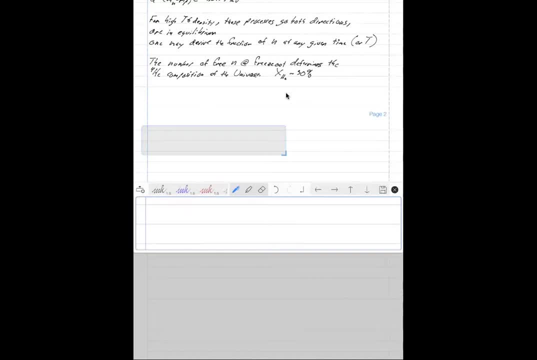 the rate of neutrons going to protons via all three channels. Now, in Weinberg, Weinberg represents the rate of going from neutrons to protons in all three channels. with this equation, I'm going to write down this interval. I'm going to write down this interval. 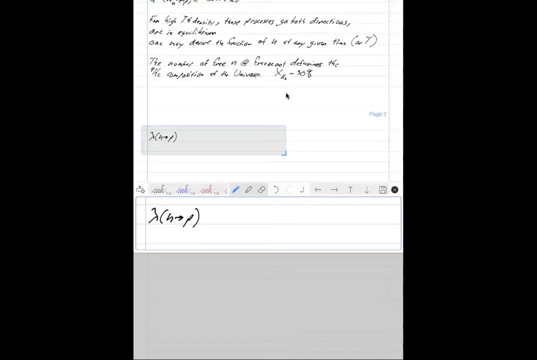 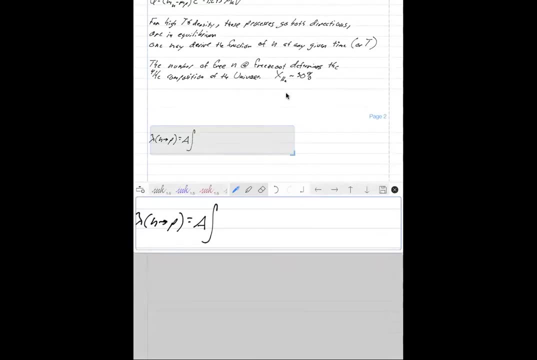 And then we're going to. we're going to see where this interval comes from. Okay, so first I'm just going to write it down: A times: integral of one minus me, squared over q, plus little q squared to the one half. I haven't even defined what little q is yet. 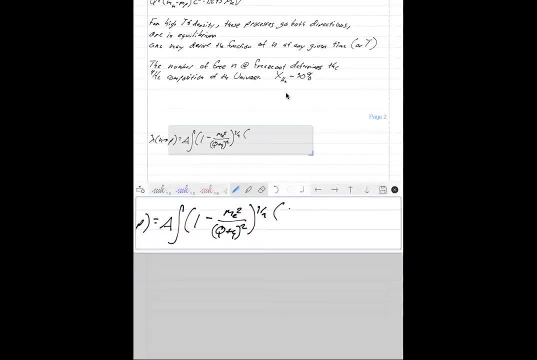 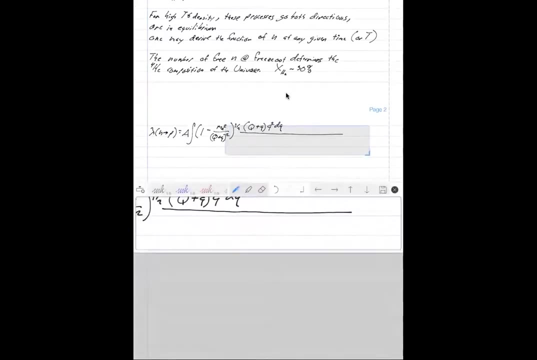 I'm just going to write it down first. And then we have capital Q plus little q, q squared dq all over one plus exponential of minus mu over kt, where that's mu is the chemical potential, and then one plus exponential of q plus little q divided by kt. 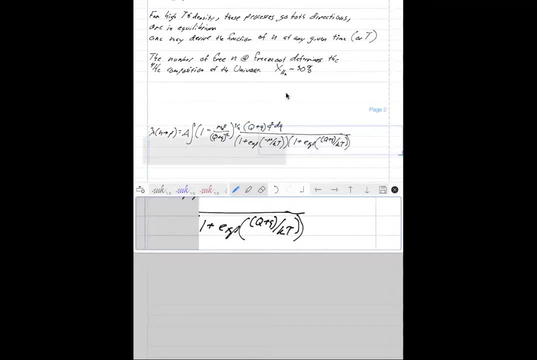 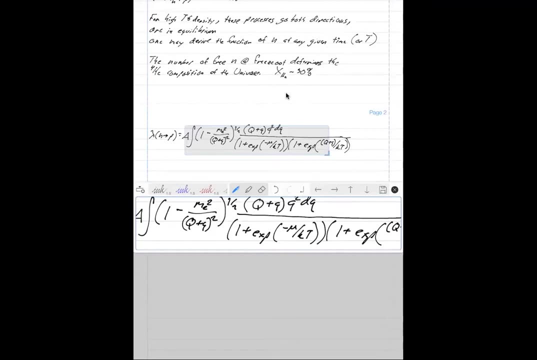 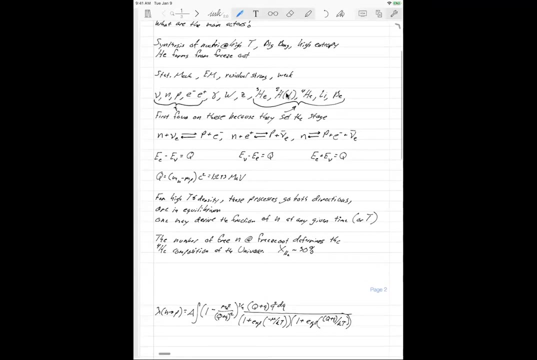 Now this seems like a complicated integral. Why do we write it down in such a way? It's really in the. by writing it down in this way, we're able to incorporate, incorporate all three of these rates of going from neutrons to protons. 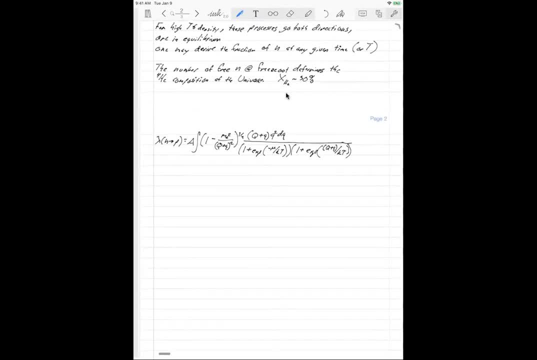 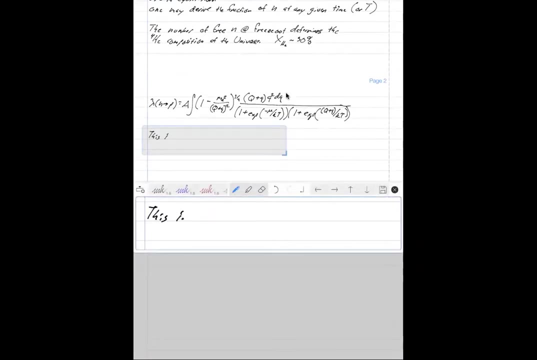 into one integral expression for the rate of going from neutrons to protons, And it's that mathematical trickery that is useful in calculating these rates. Okay, so once again, this integral represents the rate of neutrons to protons via all three channels. 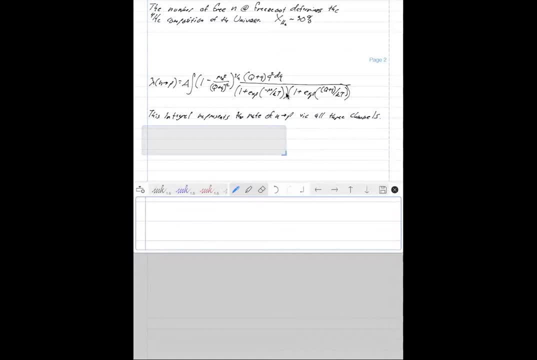 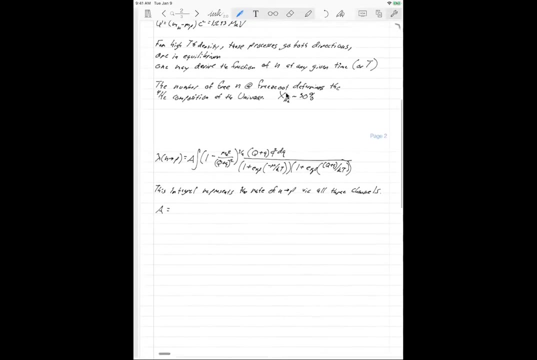 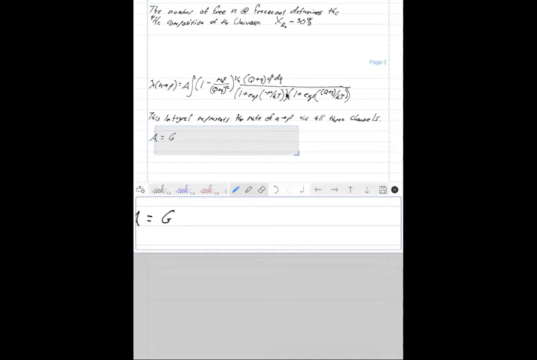 All right. And this A is is a constant that represents these are all weak interactions here And these three equations, those are all weak interactions And so A is a constant that represents the weak interactions I'm not going to, so here is: 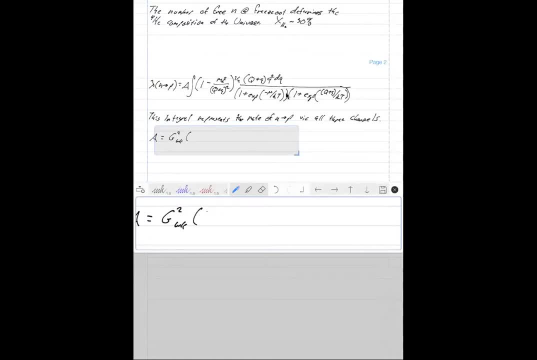 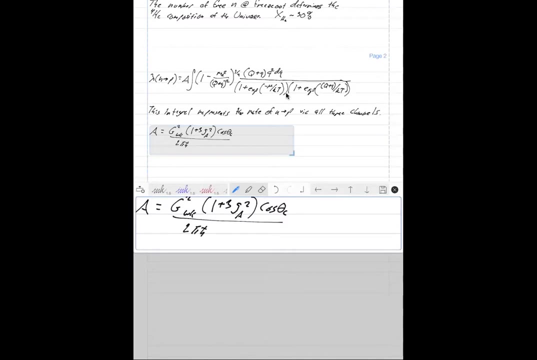 the weak interaction: constant squared One plus three GA squared cosine: theta C divided by two pi H bar, two pi cubed H bar. Now I'm not going to. this is not a nuclear physics course, So I'm not going to go into the details of 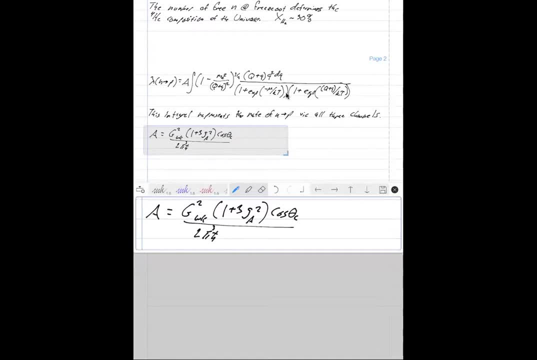 where each of these terms come from. They all have their own interesting aspects. I'll just say that A represents the scale or the strength of the weak interaction, And you can look up what each of these are on your own For the purpose of this class. 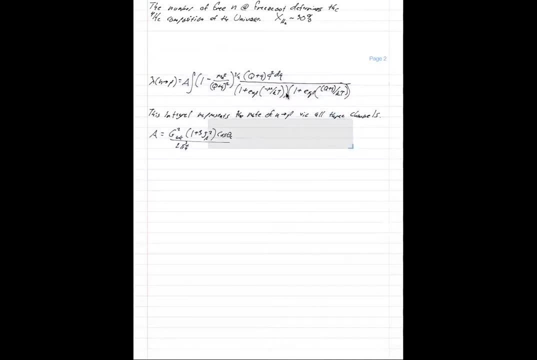 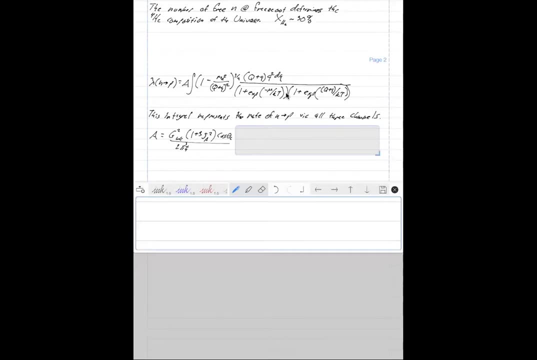 and the purpose of this math. Now, this integral will go from minus infinity to infinity, But it turns out that there are three regions of this integral that represent each three of these equations or rates or channels. And so when we integrate from minus infinity, 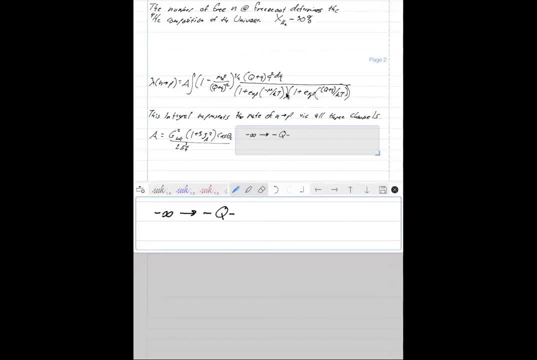 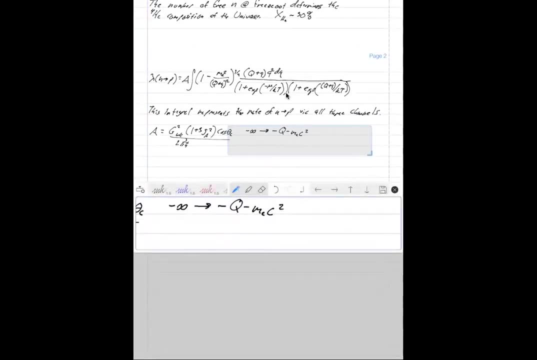 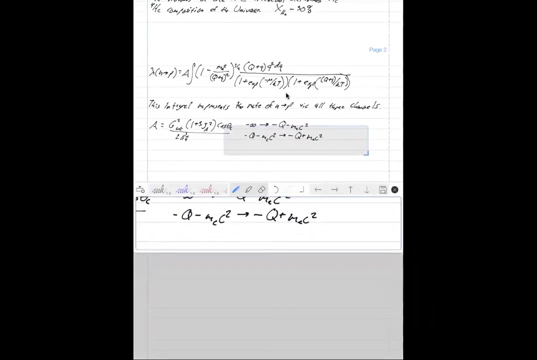 to minus Q minus M E C squared. that represents one of the equations We do: minus Q to minus M E C squared. to minus Q plus M E C squared. That represents another equation. And then when we go from minus Q plus M E C squared. 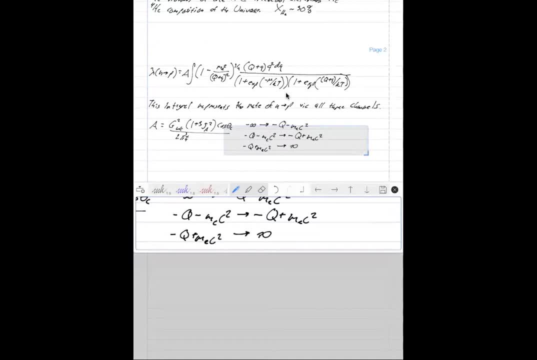 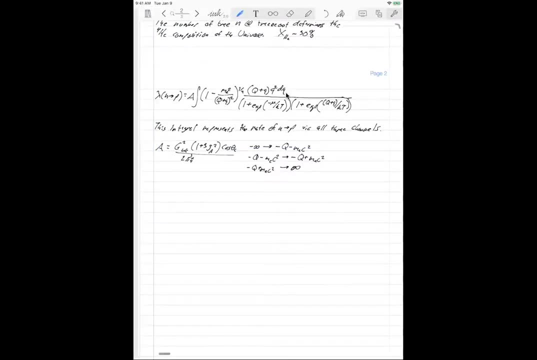 to infinity. that represents the third channel, or the third equation. And so in that way, in this way, this one integral, by taking the integral from minus infinity to infinity, represents all three channels through this funny parameter called Q. Okay, so let's. 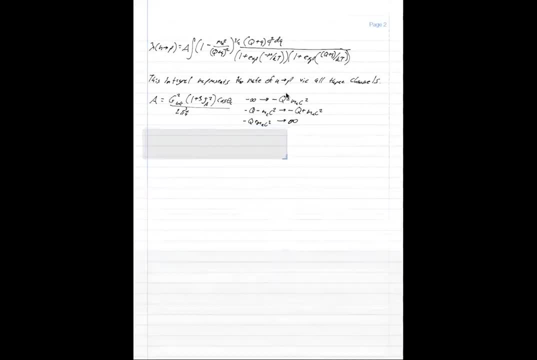 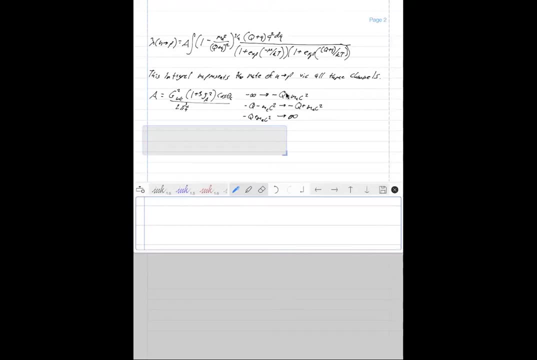 let's figure out. what is this? What was Weinberg? Why did Weinberg do this? How was Weinberg able to do this? To write down this, this rate, in one compact form. So we're going to do this. Let's do one example. 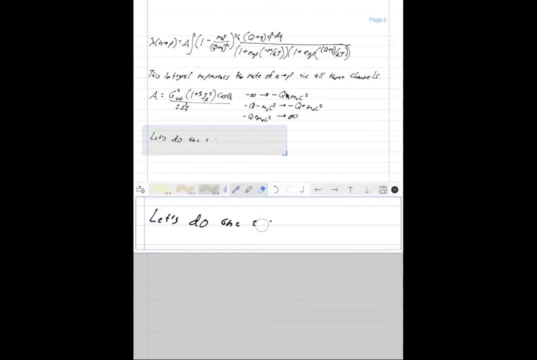 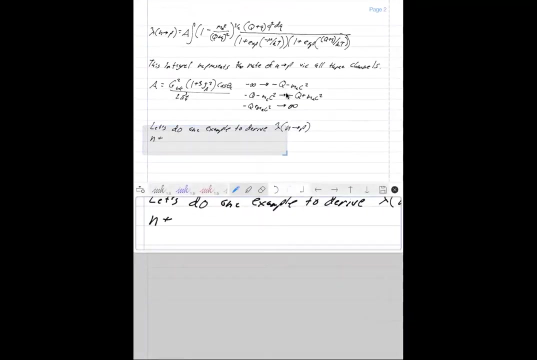 Instead of doing all three, we'll just do one example To derive this rate of going from neutrons to protons. Okay, and we'll. we'll take this one. We'll go from N plus positron goes to a proton plus the. 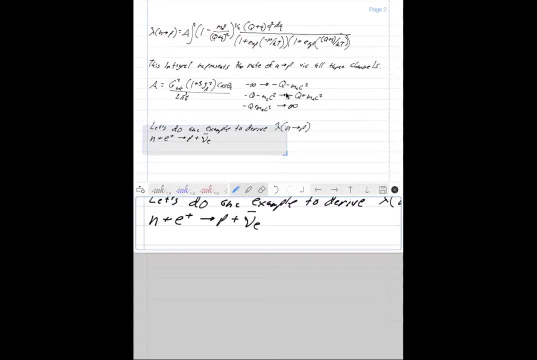 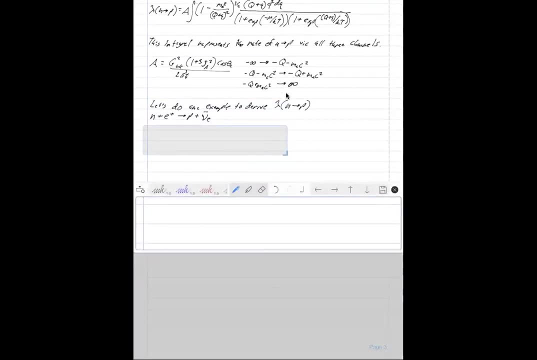 anti-electron type neutrino. Okay, So the cross section for this interaction, The cross section for this interaction is two pi h bar cubed times the same, a constant. So it gives us the scale of the weak interaction And then the energy of the neutrino. 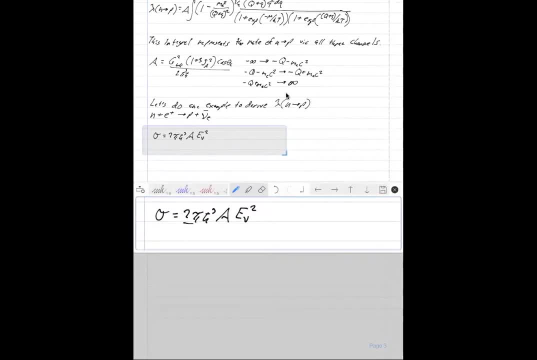 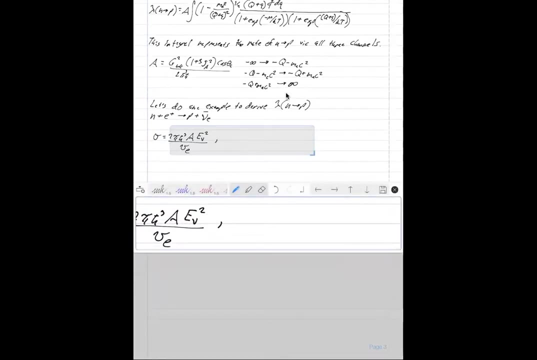 squared, divided by the velocity Of this lepton, And in this case it happens to be the positron. All right, The other thing that we need to consider is we need to consider the number density of the lepton In this case. 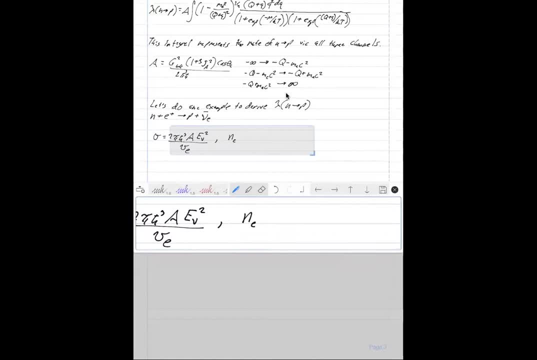 it's the positron, And so I'm going to say the number density of this positron is PE, or that's momentum, And it's a function of temperature. So it's a function of these two things. So it's a function of these two things. 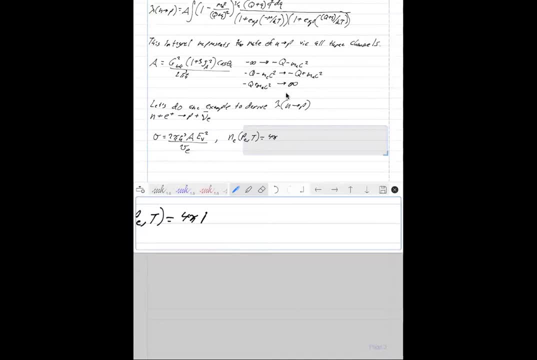 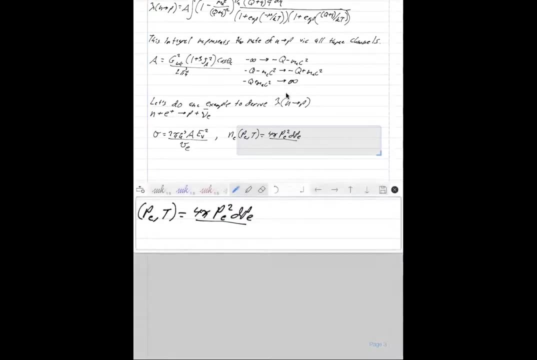 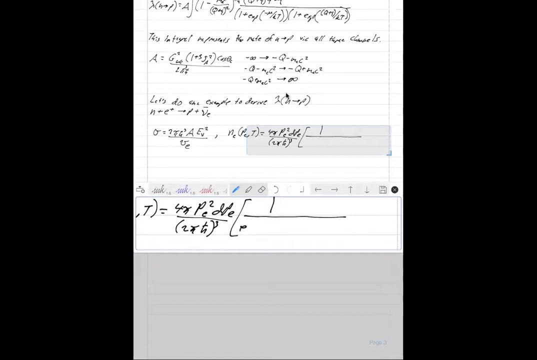 This is equal to four pi PE squared, DPE over two pi h bar cubed, and then times this one over exponential factor- because we're dealing with fermions Exponential- and then the energy of the electron divided by KT plus one. All right, 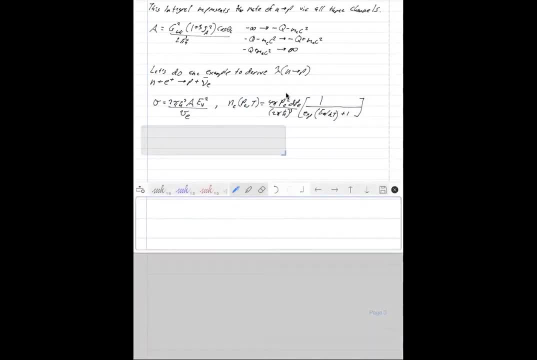 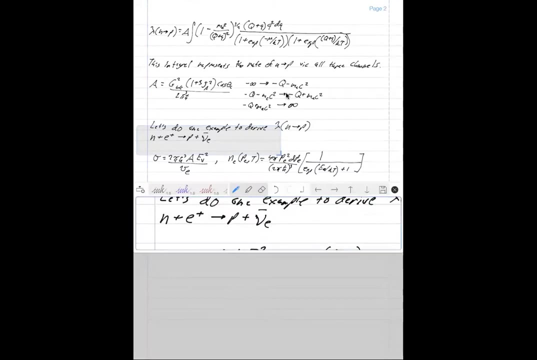 That represents the number, density of, of these leptons, In this case positrons. Okay, So now we're going, we're looking at this equation and we see that we're going to capture a positron onto the neutron. that produces a proton. 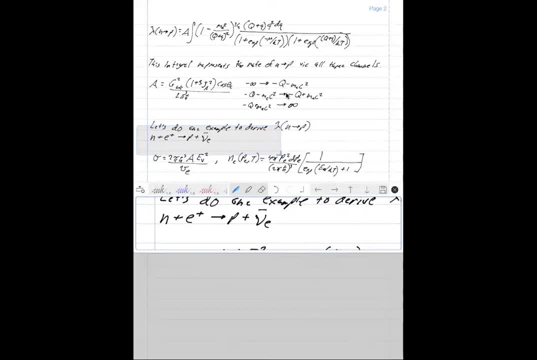 And then it's going to produce a neutrino. Now this reaction can only happen if all of the states for the neutrinos are not occupied. If all of the states are occupied, then of all, if all the quantum states are occupied, then you can't fill those states. 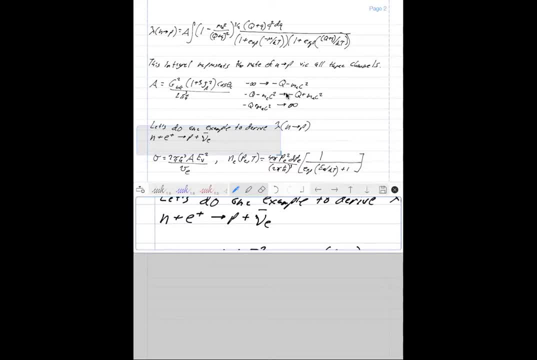 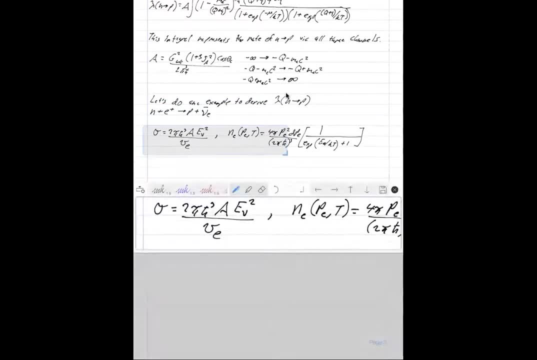 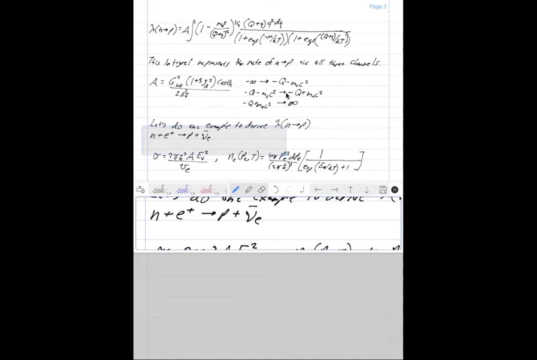 and this reaction can't happen, And so this is called blocking, And so we need to estimate what is the blocking for this reaction. So, in other words, if there are very few neutrinos in the possible states, you're likely going to have this reaction. 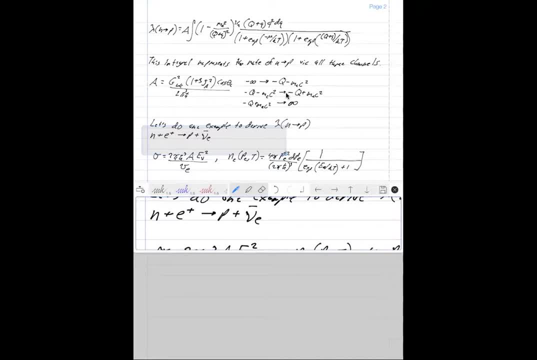 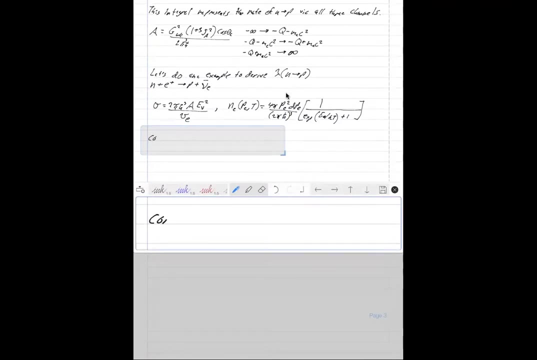 However, if most of the states for the end state neutrino- have been occupied, then it's unlikely that this reaction will go forward. So we need to consider what is the blocking. so we need to consider the fraction of unoccupied states for the anti-. 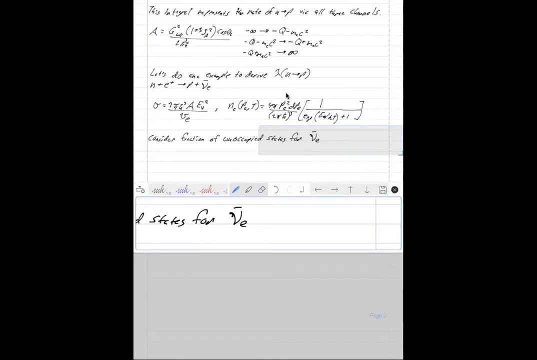 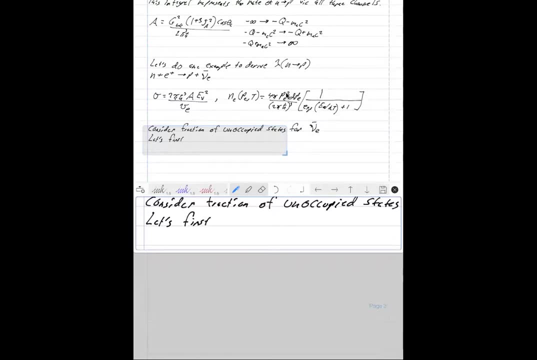 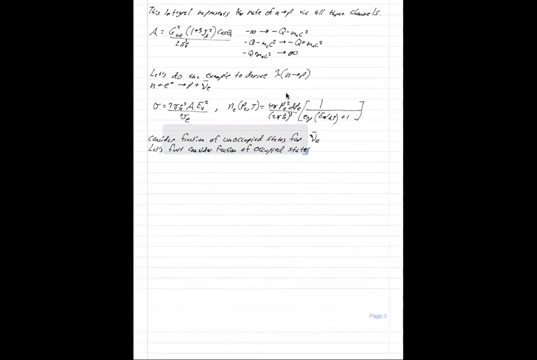 electron type neutrino. So let's first consider fraction of occupied states And once again, the reason we're doing this is the ability for this reaction to proceed is proportional to the fraction of unoccupied states. If the fraction of unoccupied states is zero, 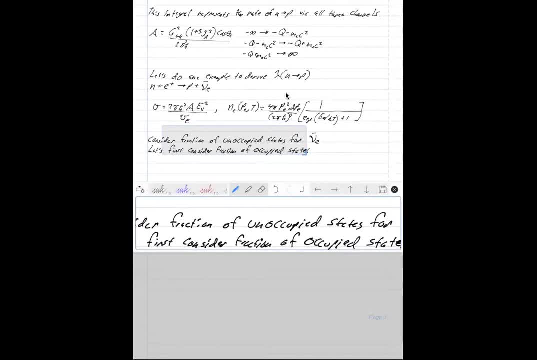 then this is not going to happen. There are no unoccupied states, because we're dealing with fermions. You cannot have more than one fermion in each of the states. Okay, So let's first consider the fraction of occupied states, That is. 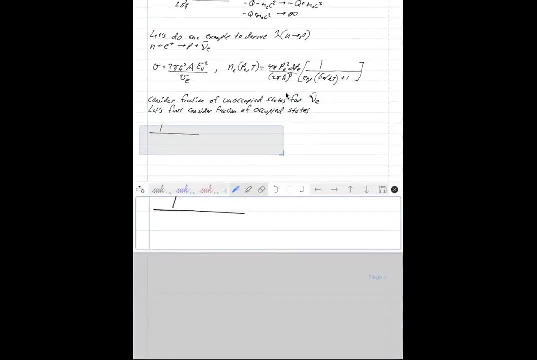 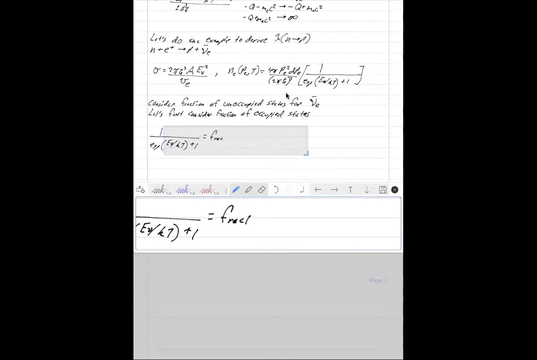 for a fermion, the fraction of occupied states is one over the exponential of e nu divided by kt plus one, This is equal to the fraction of occupied states F zero. I'm going to call it F zero Now. the fraction of occupied states. 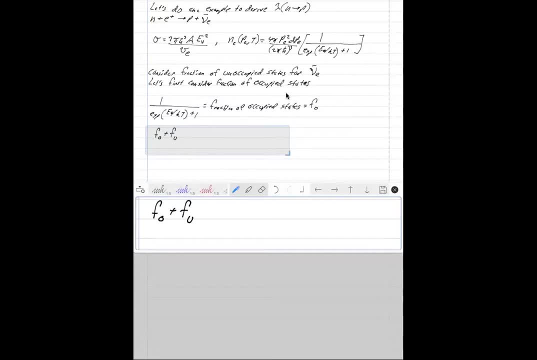 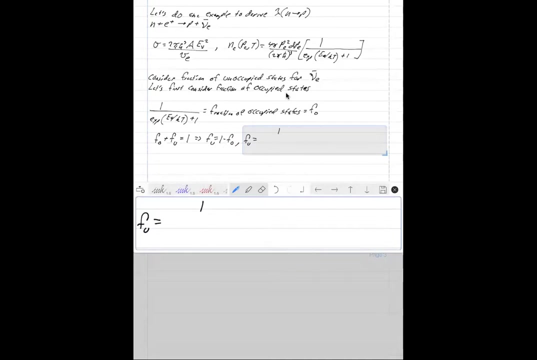 plus the fraction of unoccupied states is equal to one. All right, So now we have that the fraction of unoccupied states is equal to one minus F? o. Therefore F? u, after a little bit of algebra, is equal to one over. 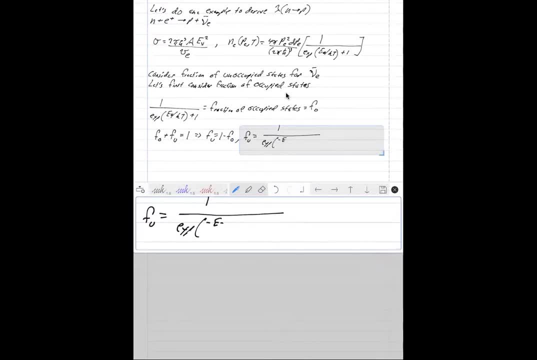 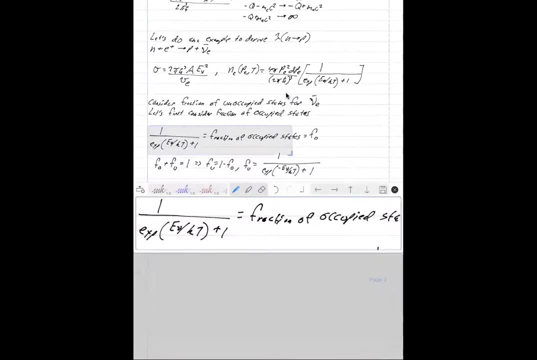 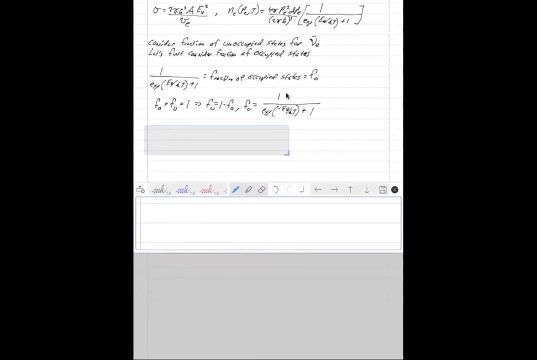 exponential of minus e nu kt plus one. So this is similar to the fraction of occupied states, except there's a minus sign in the exponential. that's in the bottom, And if I recommend that you pause the video here if you'd like. 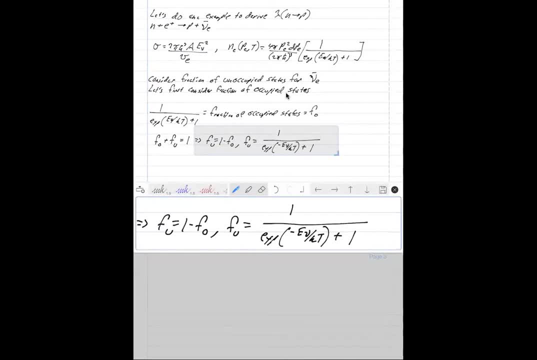 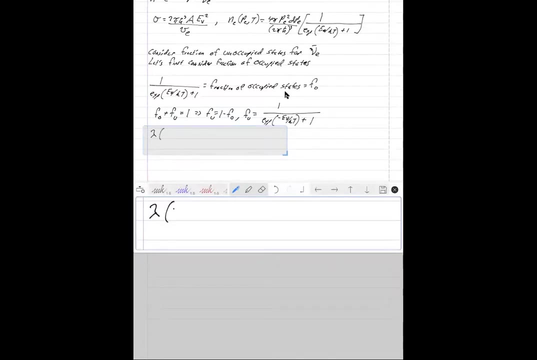 to derive, just to make sure that that is true. Okay, Now, now let's calculate the rate, The rate of this reaction happening: a neutron capturing a positron, producing a proton plus a neutrino, that's electrotype. 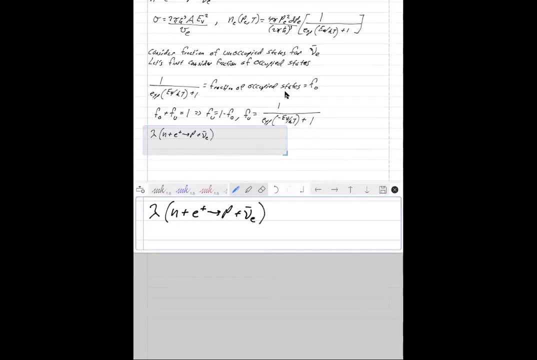 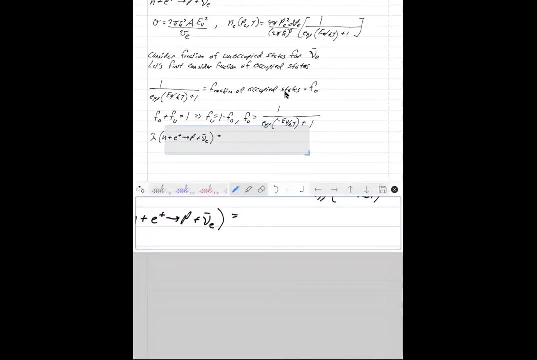 has to be anti to balance this equation. This rate is equal to well. it's proportional to the number. density of the positrons is proportional to the cross section, the velocity of interactions for the positron. And then only this will only occur. 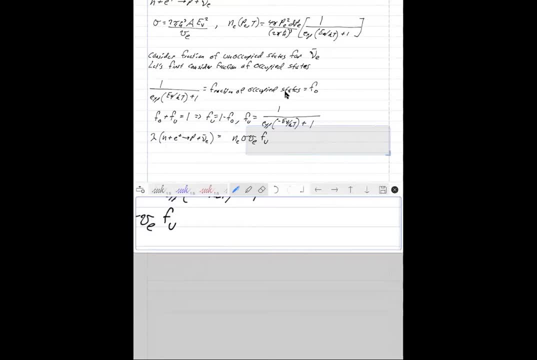 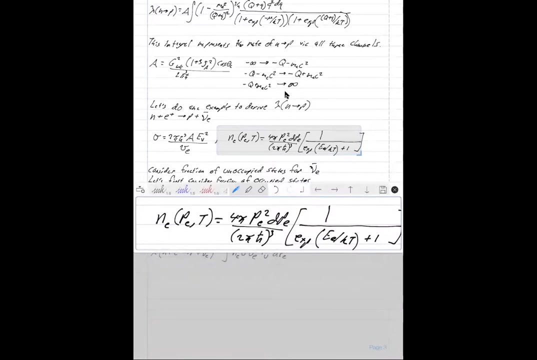 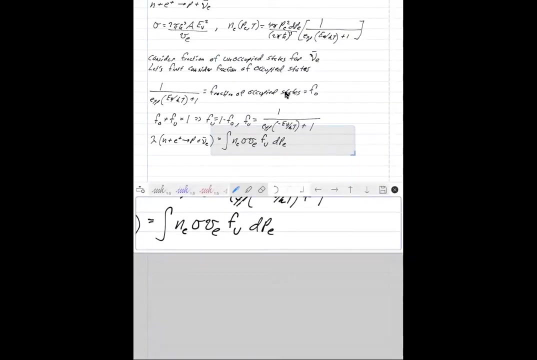 for the fraction of unoccupied states that are available, And we're going to integrate this over all of the possible momenta. Okay, remember, this density that we wrote up here is in terms like per momentum interval. Okay, So now. 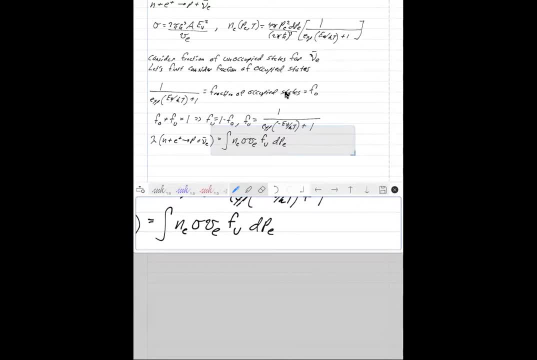 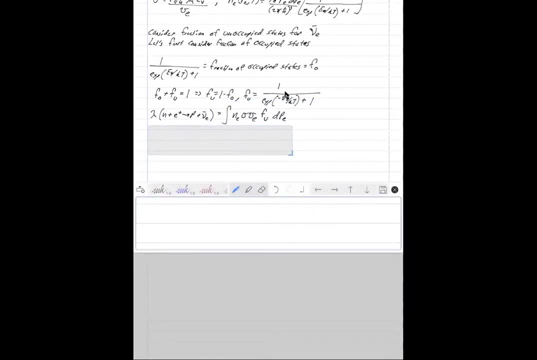 now we need to. we have expressions for each of these: the density, the cross section, the velocity and fu, And if we plug this in, we get a and we're going to integrate the momentum from zero to infinity And we have. 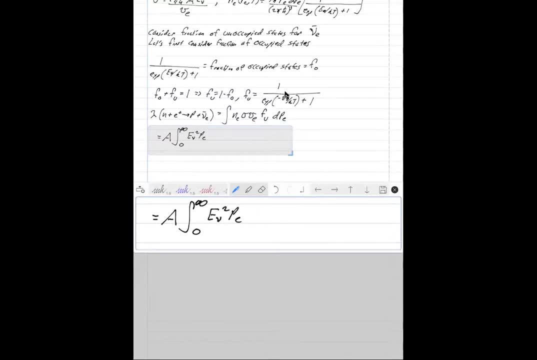 e, nu squared p, e squared times one over exponential e. energy of the electron divided by k, t plus one, And then that came from the from n, e, And then we have the fraction of unoccupied states, which is one over exponential. 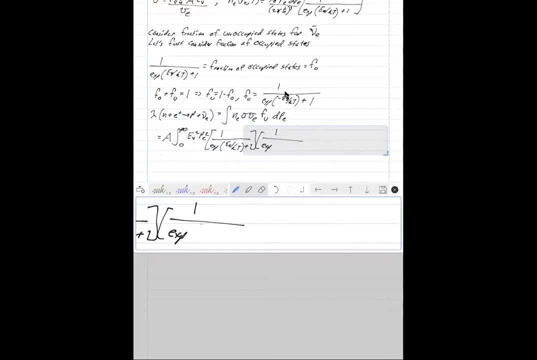 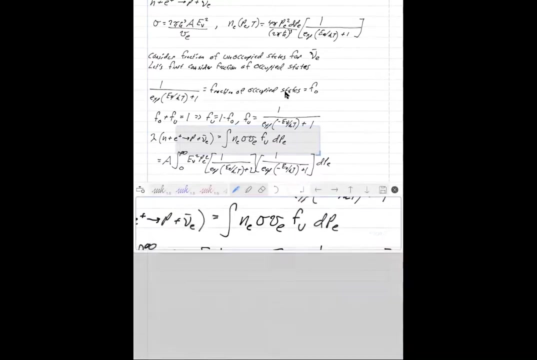 oops, let's do a parentheses here. So minus e nu divided by k t plus one, And then d p e. Okay, So what we did is we took our density n e plugged it into here, the cross section. 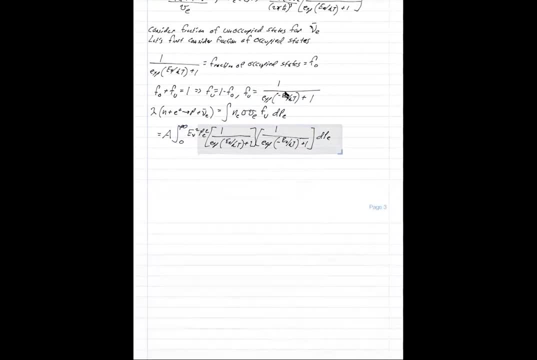 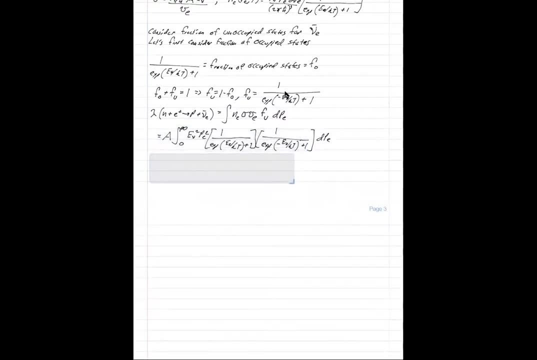 v, e and then f, u, And we end up with this integral here And we're integrating over all possible momenta for the lepton, which in this case is a positron. Okay, Now, here comes the trick In order. 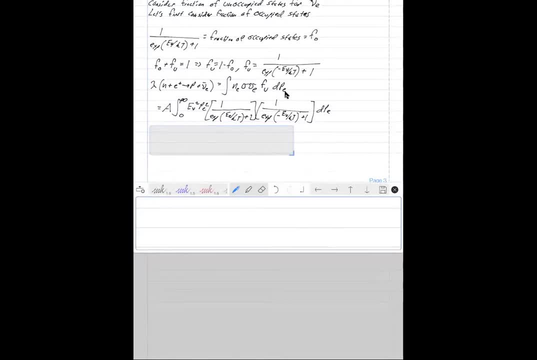 we're going to rewrite this, We're going to do some variable substitution so that we can rewrite this And then the we'll have a similar form for each of the three equations. So if we let q equal minus the energy of the neutrino, 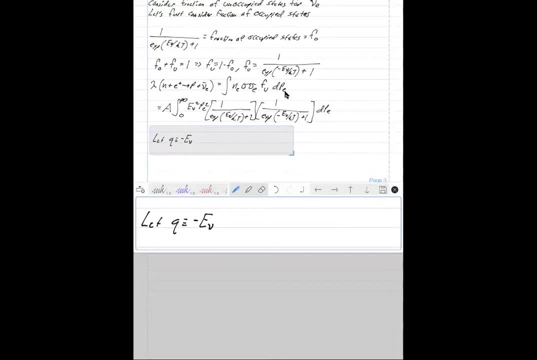 and for this particular reaction, the minus the energy of the neutrino is equal to minus q, and then minus the energy of the lepton. All right, This is the variable substitution that we're going to do Now. it may not seem obvious to you. 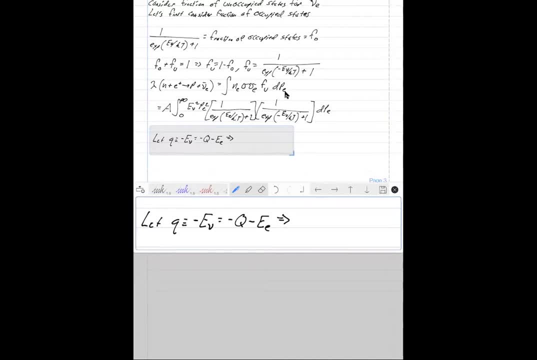 It's like: okay, fine, How's that going to work? It will lead to a form of this: that when you do a similar variable substitution for all three equations, you see the same type of integral, In fact the integral that we wrote up above. 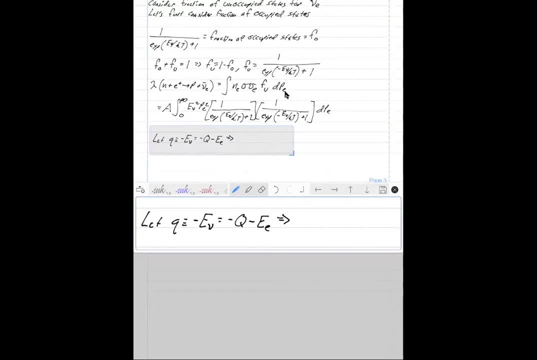 And I'm just going to work through doing this variable substitution for this one particular case for one of these equations. All right, So now let's go ahead and square q, So q squared is equal to the neutrino energy squared right. 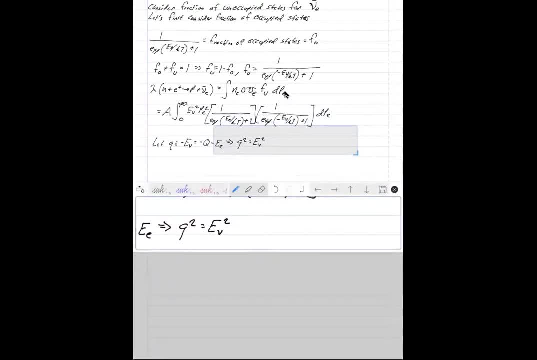 We have the neutrino energy squared up here, So that's why we did that. We wanted to find q squared, And we have that. This is another expression that will be useful in the substitution. If we rearrange this, we have q. 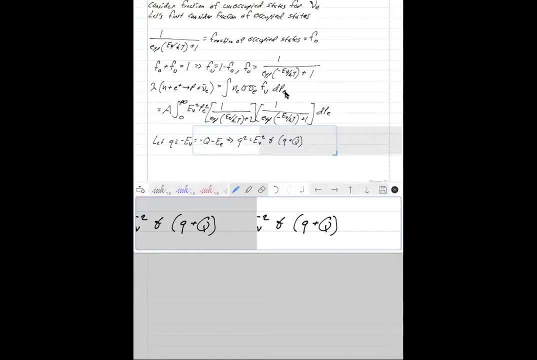 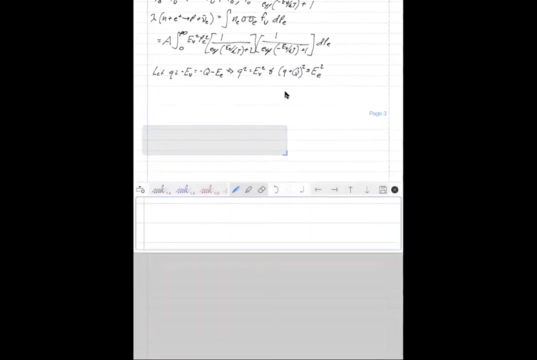 little q plus capital, Q, squared is equal to the energy of the lepton squared, In this case as a positron. Okay, So now we've done this variable substitution of q, which apparently is related to energies. All right, We're going to be integrating over q. 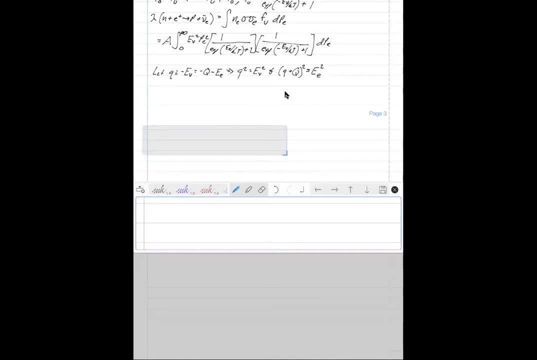 instead of momentum. So we need to find dq in terms of pe. So if you would like to pause here and work this out yourself, feel free to do that. And now we'll compare to what I have found. So dq is minus one half. 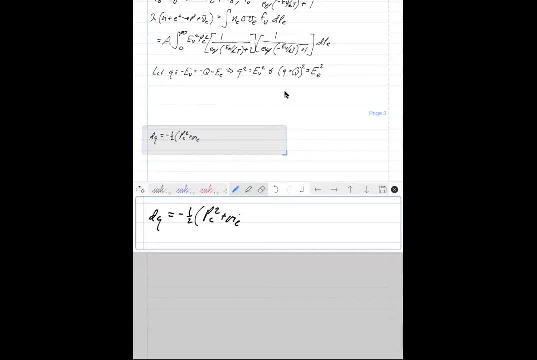 pe squared, So that's the total energy of the lepton plus me, squared to the minus one half, So that's the total energy of the lepton times. two pe, dpe And the twos cancel. The two and the one half cancel. 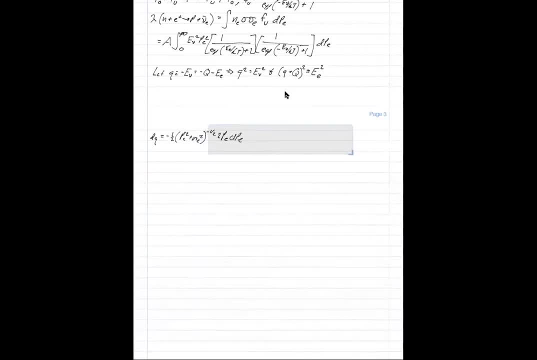 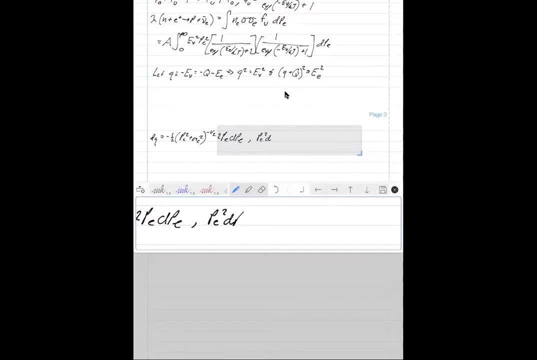 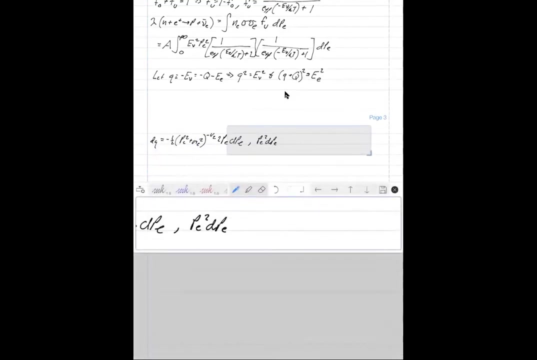 All right, And so we have. if we rearrange, we have that pe squared, dpe, which is what appears in the integral equation up above. Up here we have pe squared and then dpe. So rearranging this here: pe squared. 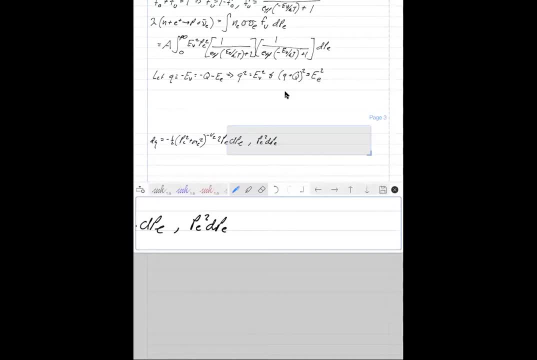 times dpe is equal to minus q, capital Q plus little q squared dq times one minus me squared. I'm obviously leaving off a c squared there, Divided by little q plus capital Q squared, and all of that to the one half. 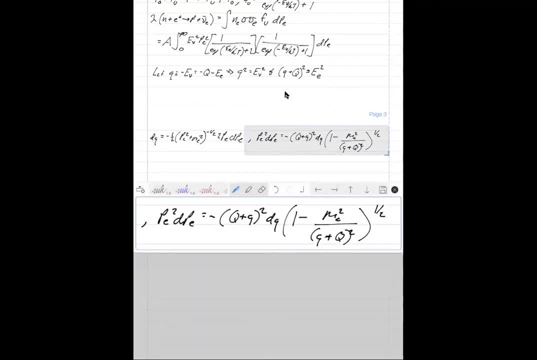 Now that may seem like okay. It wouldn't be obvious at first glance that replacing pe squared dpe with this mess on the right hand side would get you anywhere. But once again, the reason we're doing this is when we make this substitution. 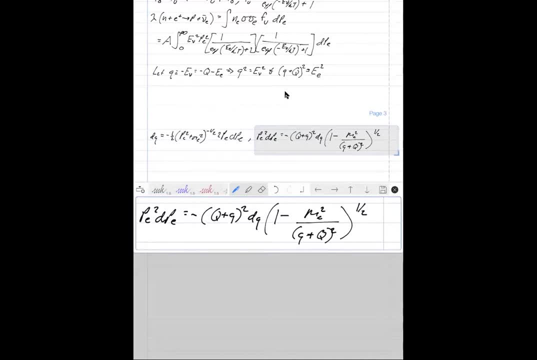 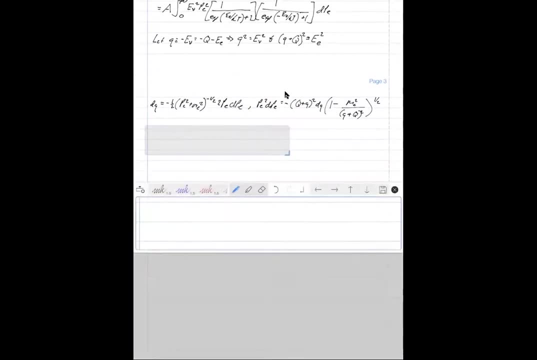 in each of these equations we get the same integral, but with, just with different limits. Okay, So let's go ahead and plug that back in. And now we have that: the the rate of going from neutrons or protons for this particular reaction. 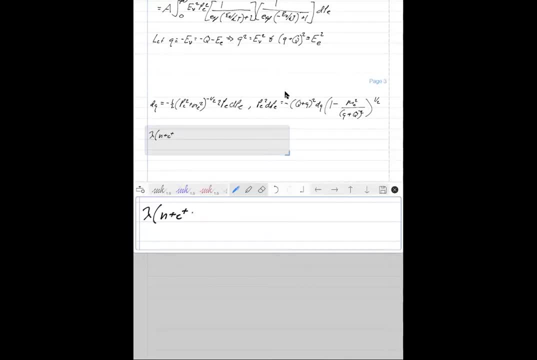 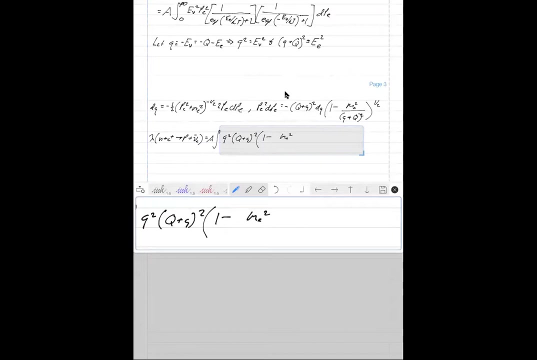 So plus a positron gives us a proton plus an electron. time neutrino is equal to a integral q squared times q plus little, q squared times one minus me, squared divided by little, q plus capital, Q squared to the one half, And then we have dq. 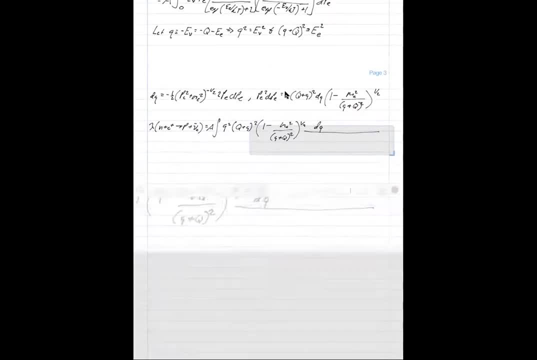 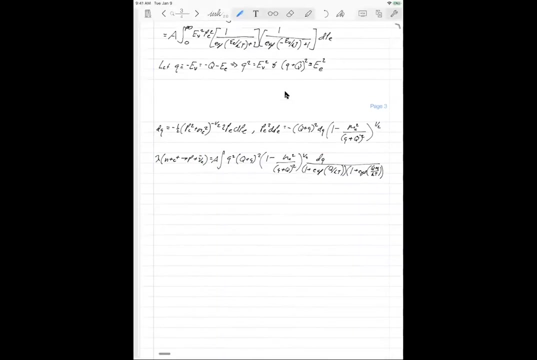 integrating over this new variable. And then we have two exponentials in the bottom, One plus exponential q divided by kt, and then times one plus exponential of capital, Q plus little q divided by kt. All right, So now we have this expression, And if 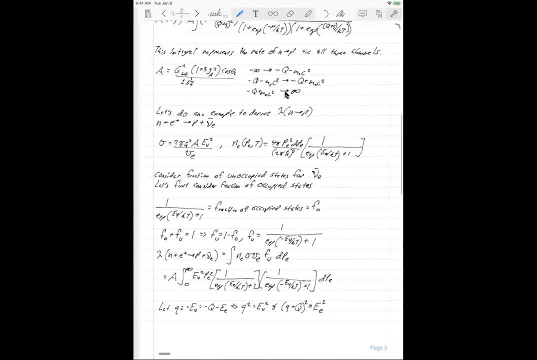 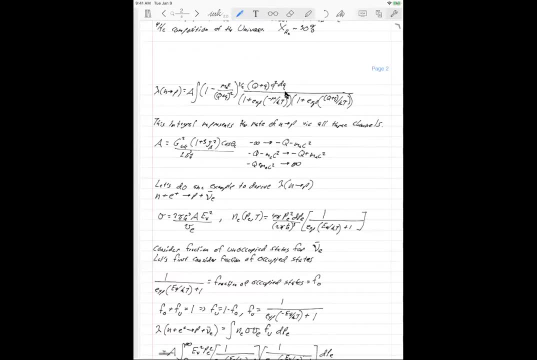 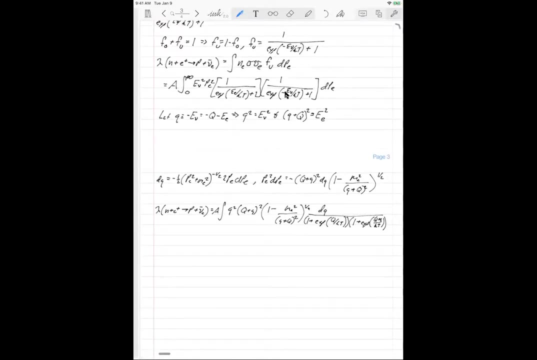 everything is done right, it should look just like this one up here. Okay, All right. So now that we have that expression, now we need to see what is this expression in terms of, or what are the limits of integration for this? Well, 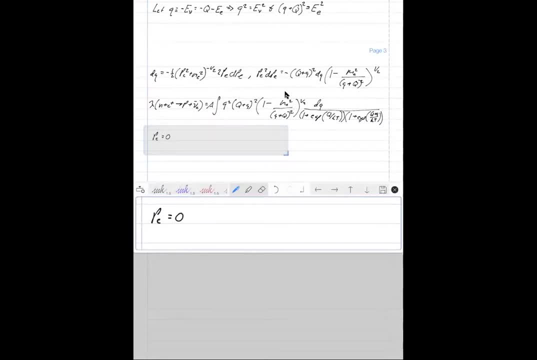 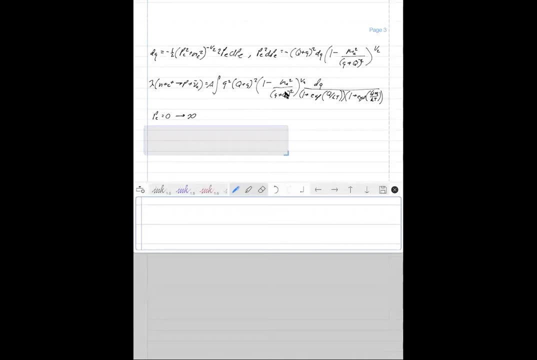 we were integrating pe from zero to infinity. Okay, Now recall that we need to figure out what are the limits of integration for q. Recall that q is equal to minus e. nu is equal to minus q. minus e little e the energy of the lepton. 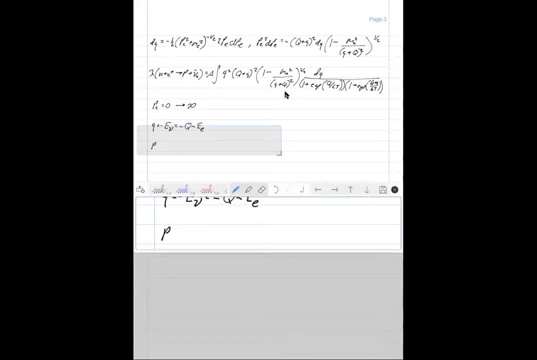 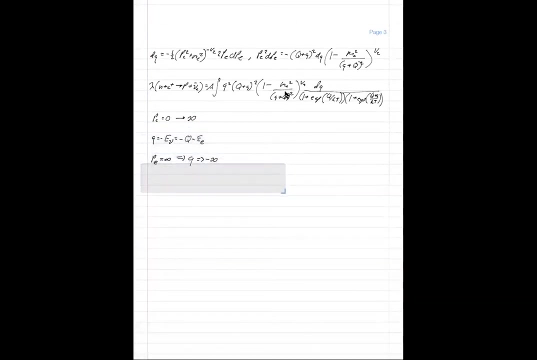 or positron. Now, when the momentum is equal to infinity of this lepton or the positron, then q goes to minus infinity. So up here, if the momentum is infinity, then e sub little e is infinity And we go, q is minus infinity. 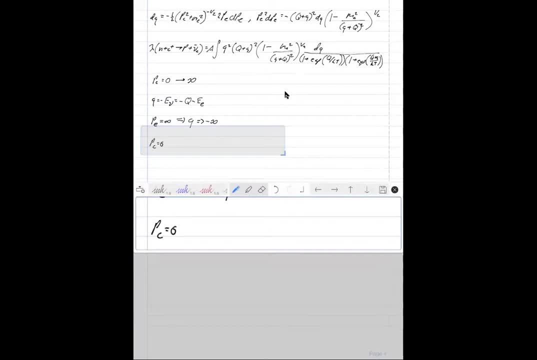 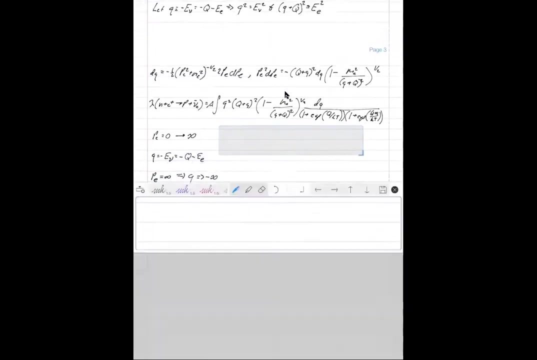 And if pe is equal to zero, then q goes to minus q, and then minus m e c, squared. And so those are our new limits of integration: We're going from minus infinity to minus q, minus m e c, squared. All right. And so now we see that. 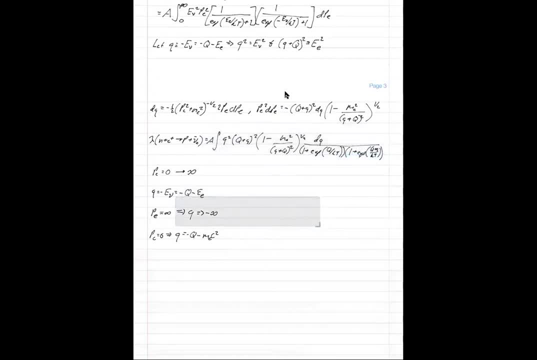 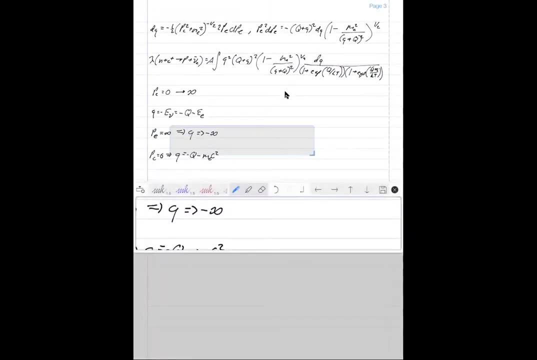 this integral of this specific form, integrated over these specific bounds here, gives us our rate for that one equation, And if we want the rates for the other equations, we just need to add those other two And it turns out you get the same integral. 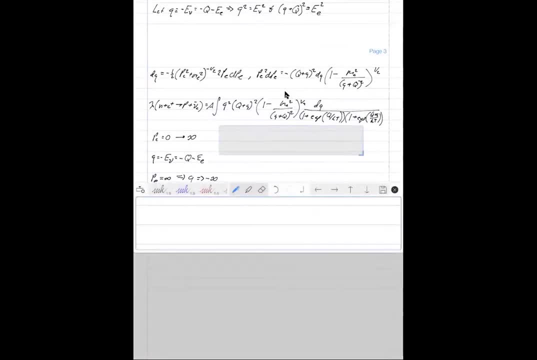 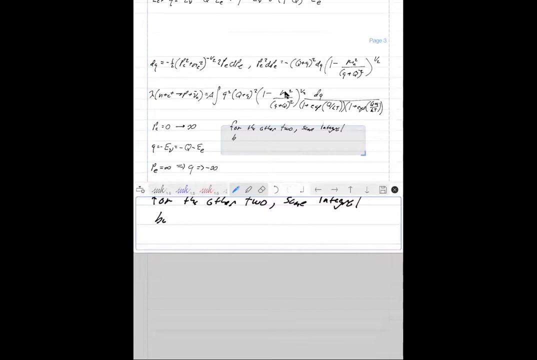 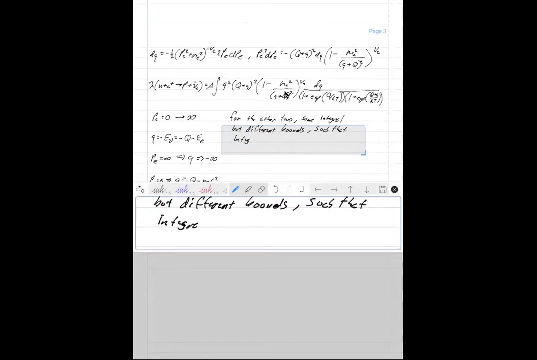 but slightly different. So we can see that the different integration bounds. So for the other two we have the same integral. There we go: Same integral But different integration bounds, But different bounds, Such that integrating q from minus infinity to infinity. 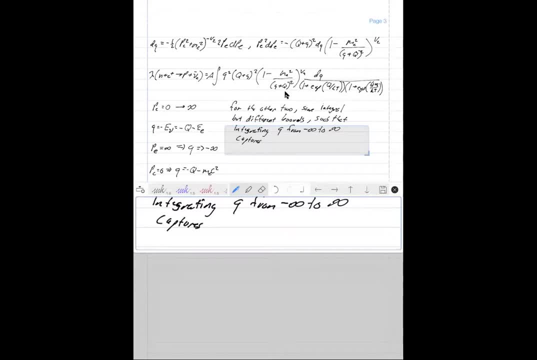 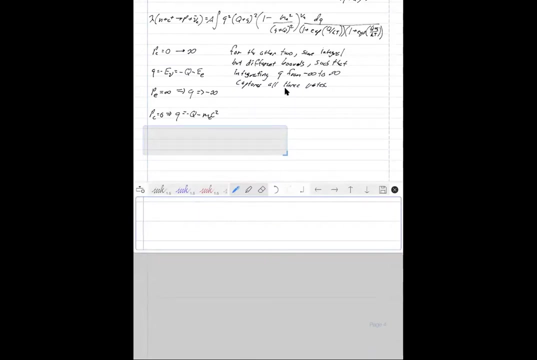 captures all three rates. Okay, All right, So now moving along. So these are the rates. To figure out what is the, the mass fraction of neutrons in the universe, we need to solve a rate equation. So the time derivative of the mass fraction of neutrons. 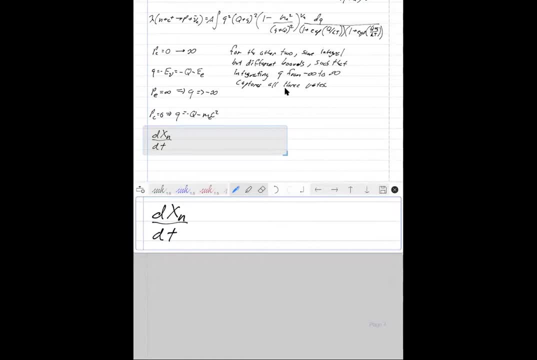 so the mass fraction of neutrons is x sub n and the time derivative d by dt is equal to well is going to be equal to minus the rate of neutrons leaving. So that's lambda n to p times the number of. 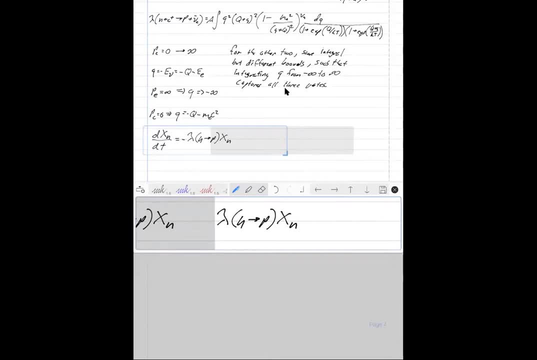 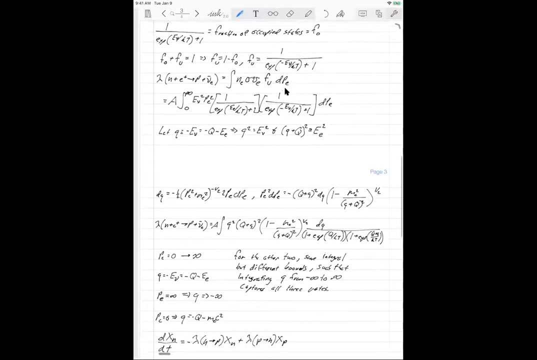 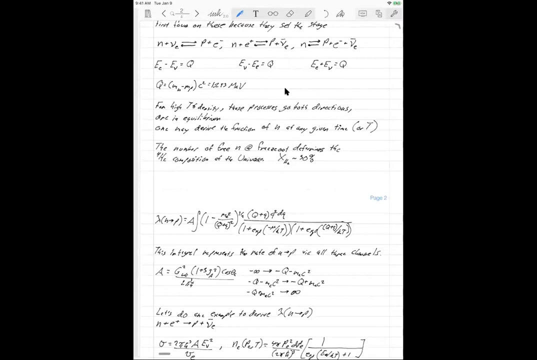 neutrons you start with, But this also increases by the rate of protons going into neutrons. So this is the rate of protons times the mass fraction of protons. So this is our balance of neutrons And we didn't derive the rate equation from going from protons to neutrons. 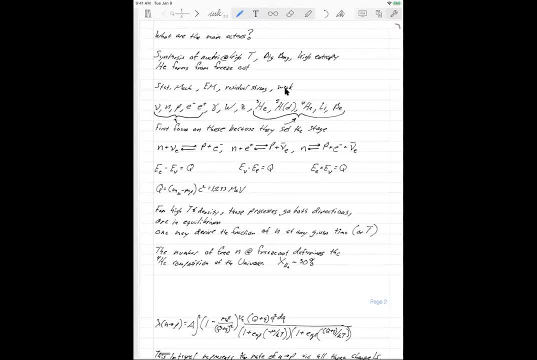 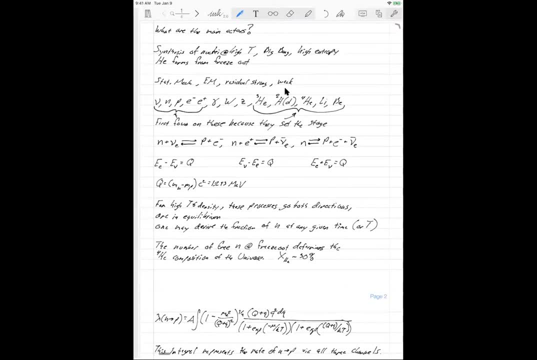 It's very similar to what we did, with one slight but important difference, And we'll get to that in a second. But it's just basically looking at the same equations and going in the opposite direction. And going in opposite direction, what you notice? that, instead of 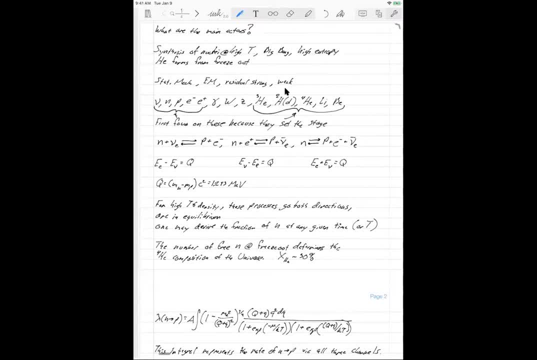 so the way I've written these equations here and here and here we're starting off with the baryon that has a higher mass going to a baryon with a lower mass on the right-hand side, And so that's going down in energy. 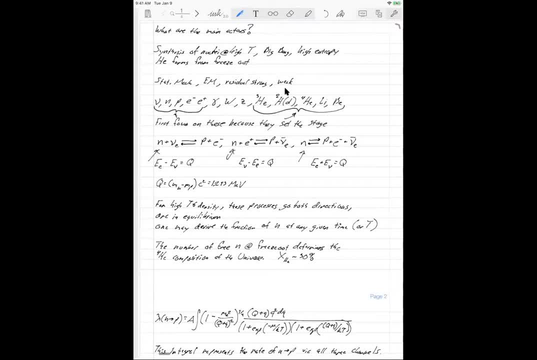 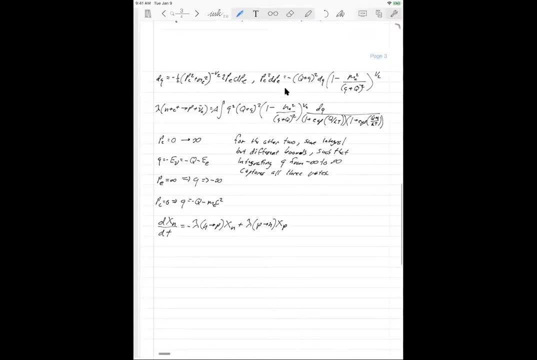 And if you go in the backward direction, you're going up in energy, You're going from the baryon with lower mass to baryon with higher mass, And that is the main difference in the rates in going the other direction. It's in fact the same equation. 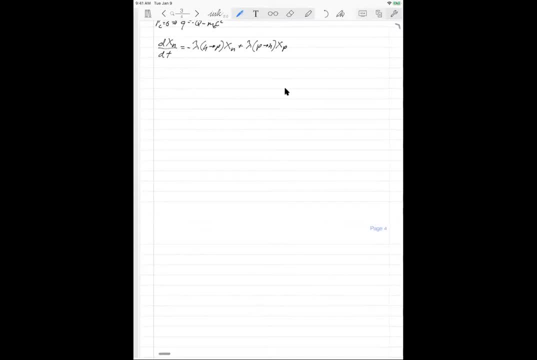 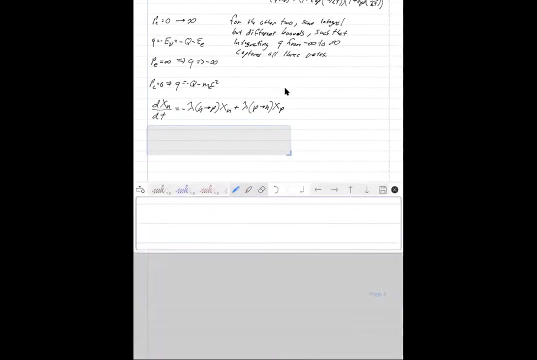 so very similar, but going the opposite direction. you're going up in energy instead of down in energy. We're going to. let's recall that the total mass fraction of neutrons plus the mass fraction of protons equals one. All right. 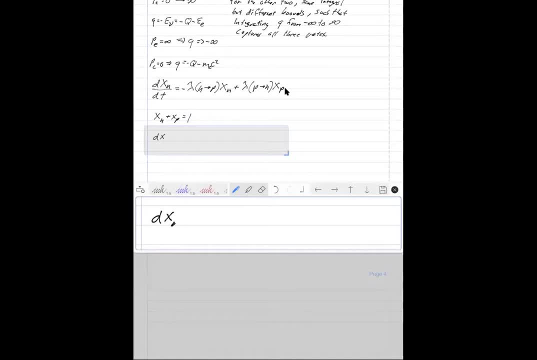 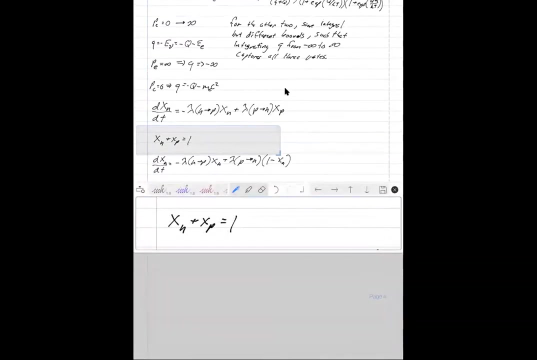 Therefore, we can rewrite dx of n by dt is equal to minus lambda going from n to p, times the number, the mass fraction of neutrons, plus lambda going from p to n times one minus xn. I'm substituting, I'm taking this equation. 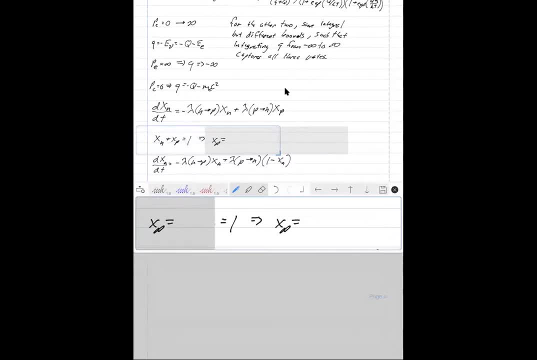 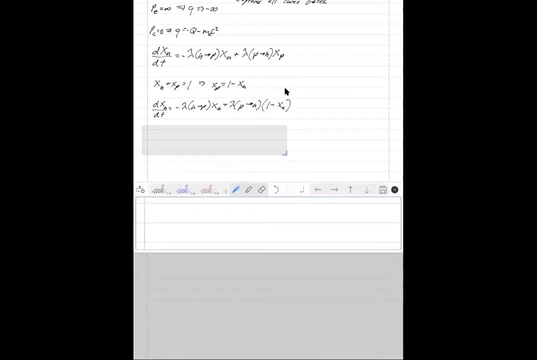 and just saying that xp is equal to one minus xn, And then we're going to plug that into here. All right, Now, in equilibrium. in equilibrium, the rates of these going both ways is roughly equal. So dxn by dt is roughly equal to zero.